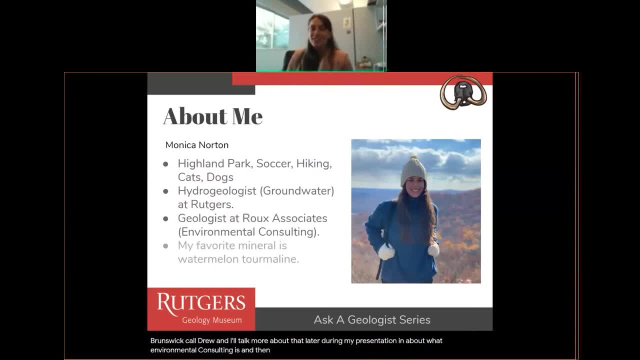 consulting is. And then last, just a fun fact, my favorite, or just a fact about myself: my favorite mineral is watermelon tourmaline, And it looks like that. And watermelon tourmaline is a bi-color mineral, meaning it can have more than one color, And in this case, 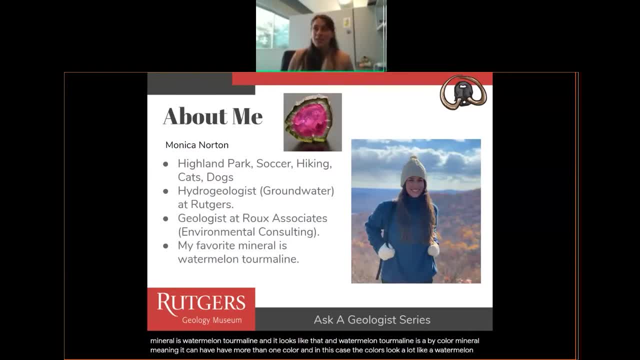 the colors look a lot like a watermelon, And actually sometimes the colors are reversed, where the pink is on the outside and the green is on the inside, And that's called anti-watermelon tourmaline. Okay, so to begin, let's just first talk about what even is. 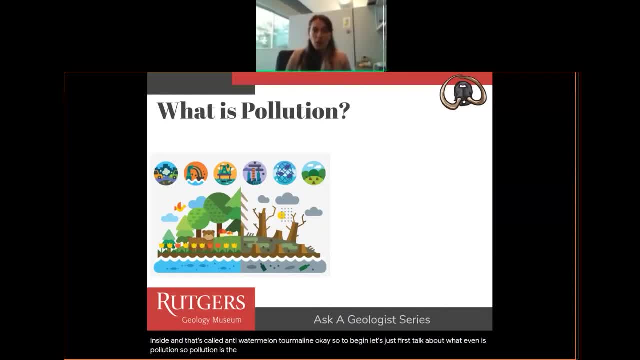 pollution. So pollution is the introduction of harmful materials into the environment, And so what we call pollutants are called pollutants, And they can be natural, like volcanic ash, which impacts air quality. Also could be natural, like wildfires, which you know, like the ones. 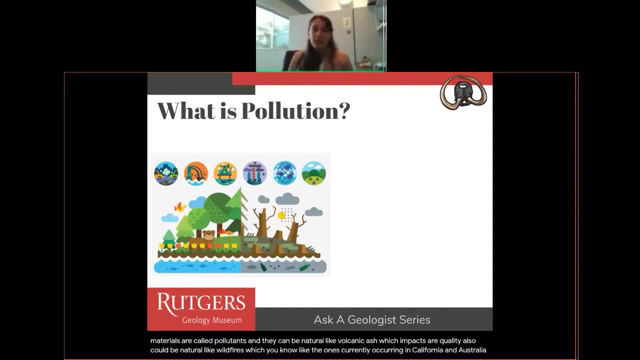 currently occurring in California and Australia and Siberia. That's also like a natural pollutant that can impact air quality, for example, But they can also be man-made, which means they're created by human activity, like trash or chemicals produced by factories And ultimately pollutants. 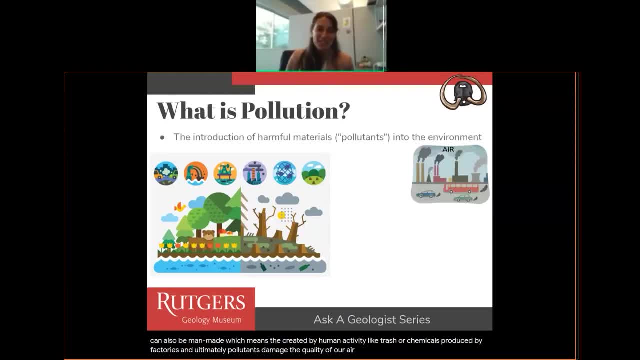 can damage the quality of our air. Oops, I didn't put the definition there, Sorry. They can damage the quality of our air, of our water and of our soil. And there are other kind of pollutants like noise and light, And I'm not really going to be focusing much on that today. I'm mainly going to 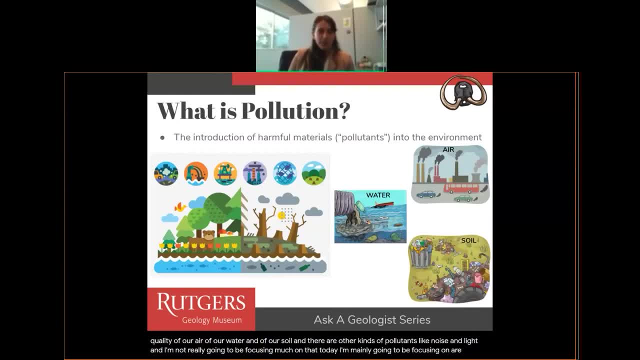 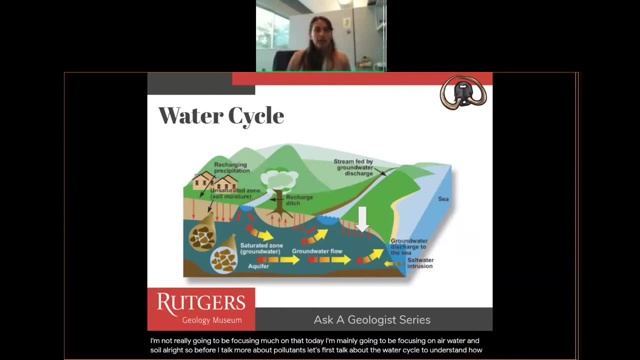 be focusing on air, water and soil. All right, so before I talk more about pollutants, let's first talk about the water cycle to understand how the air, water and land are all connected. So you all here should be pretty familiar with rain, and maybe you even know the fancy word for. 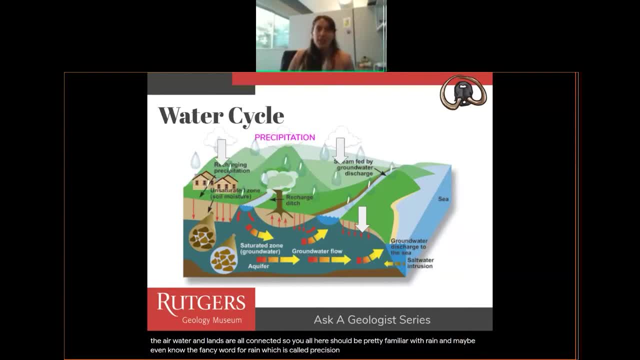 rain, which is called precipitation. So if you were a drop of rain falling onto the land, your number one goal is to make it to the lowest place that you can find, which is the ocean. So when you fall onto the land as a raindrop, you might flow down the surface of the land until you reach a 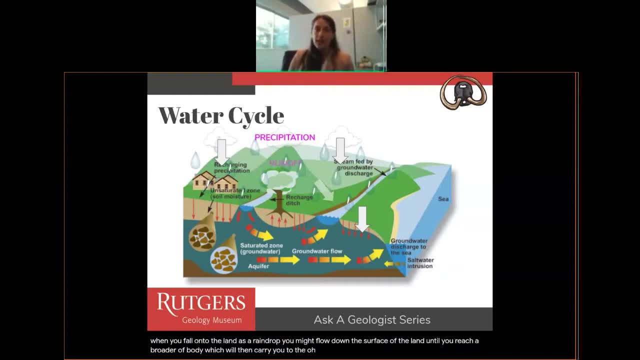 broader body which will then carry you to the ocean, And that's actually called runoff. But also you might actually infiltrate into the land and become a part of the groundwater. So you know how I mentioned before what groundwater was. So you, basically, underneath the ground there are. 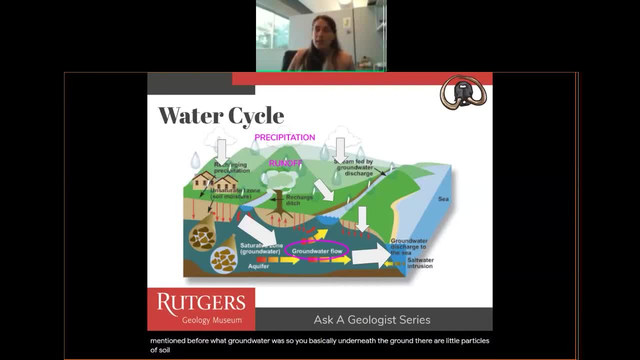 little particles of soil And in between that soil there's air. So when the water moves through those particles of soil it eventually will reach an area where it's completely filled with water And that's called an aquifer, where our stored underground water exists. So both cases, whether 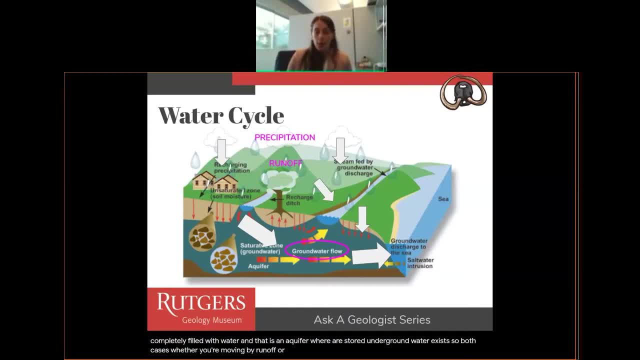 you're moving by runoff or through by groundwater flow, eventually you'll reach the ocean. And when you reach the ocean you'll evaporate back into the air, where you become a gas again and condense back into a cloud, where the whole cycle will begin again. That's why it's called a cycle. 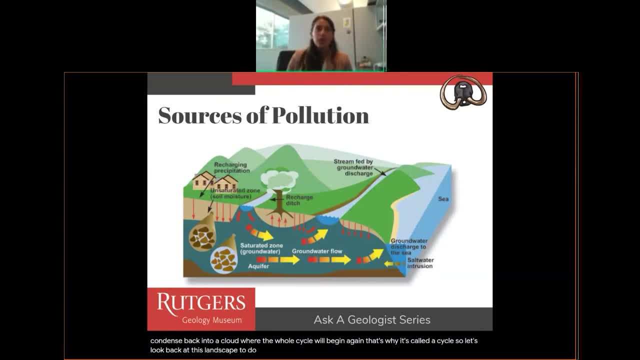 So let's look back at this landscape to determine what sort of human-related activities can contribute to pollution. All right, so let's start by building a factory. Factories release large smoke stacks, which contain a lot of greenhouse gases and pollutants that impact air quality negatively. What else? Factories also dump dirty water used. 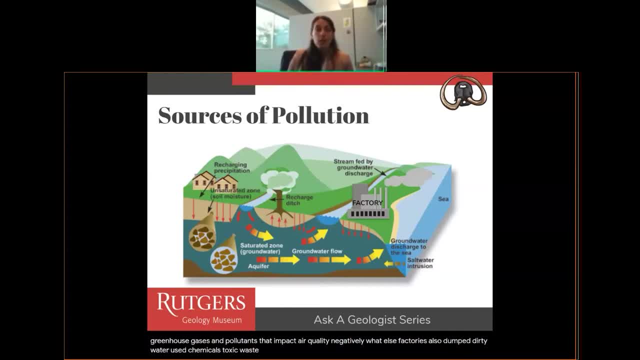 chemicals, toxic waste, and sometimes they can spill oil into the land or water, kind of like you see right over here. Okay, so these animals will come in, say, into the ocean. there's a lot of toxic chemicals inside of this, and these chemicals can then poison our groundwater. All right, what else could? 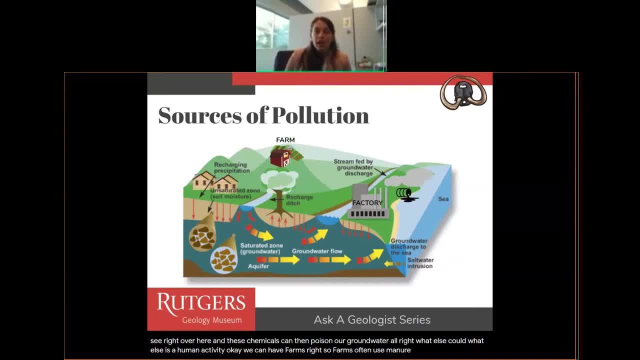 what else is a human activity? Okay, we can have farms right. So farms often use manure, fertilizer, herbicides, pesticides in order to get large crop yields, And these products actually can impact soil and air quality negatively. They contain a lot of toxic chemicals in them. Also poop from animals-. 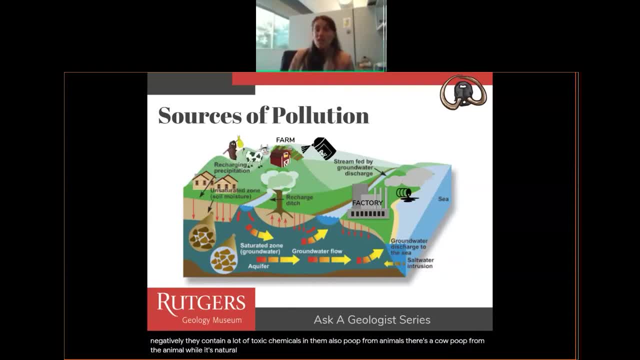 There's a cow Poop from the animal- Wow, while it's natural, it is also a pollutant and, in large quantities, can negatively impact the environment. Speaking of poop, imagine you know that the sewer lines can get damaged and they can leak and or flood, and that can actually then spread pollutants into our 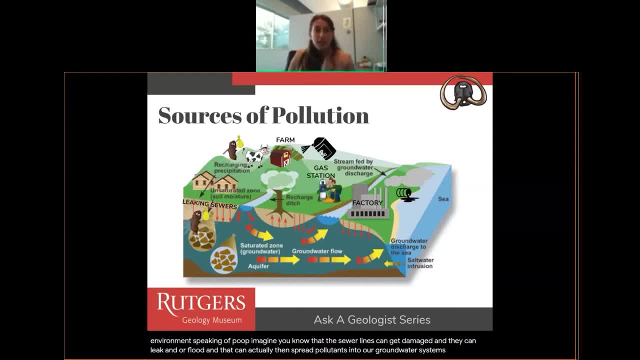 groundwater system, All right. so gas stations hold a lot of gasoline and tanks underground which, can you know, leak this harmful, these petroleum products. And you can see this guy over here is being very, very careless with this gasoline, just pouring it right all over the 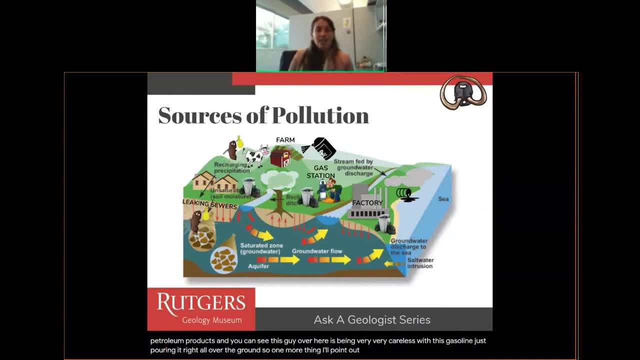 ground. So one more thing I'll point out is that humans produce a lot of trash, and a lot of that trash ends up in rivers, streams, oceans, and it can't be broken down naturally. So this is just an example of some different human activities that can exist on earth that can contribute. 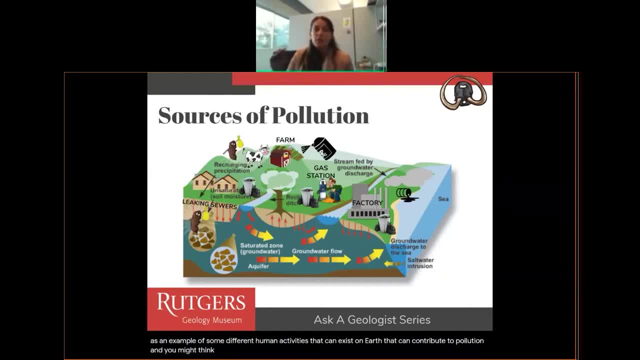 to pollution And you might think that if you were to spill some oil or drop some trash or spray some harmful chemicals in one location, that you might not be impacting anyone outside of that location. But you have to remember that there's a water cycle, there's wind, there's weather right. 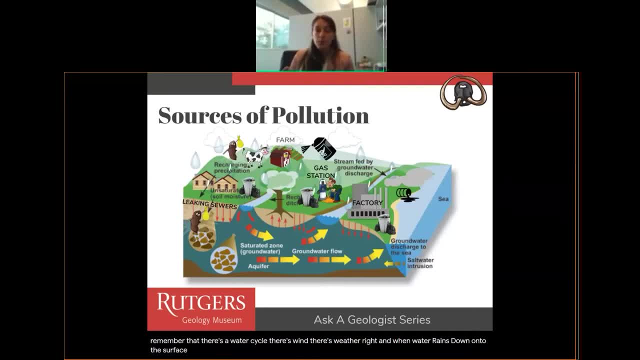 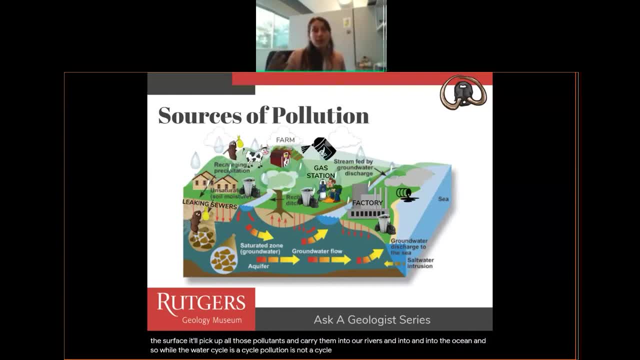 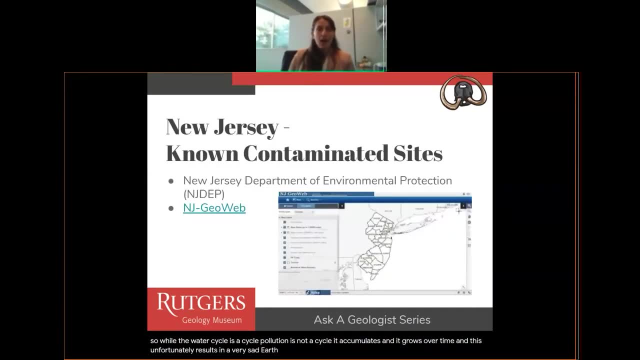 And so, while the water cycle is a cycle, pollution is not a cycle. It accumulates and it grows over time, And this unfortunately results in a very sad earth. All right, so now you might be curious whether you live somewhere that is polluted. Well, actually, the New Jersey Department of 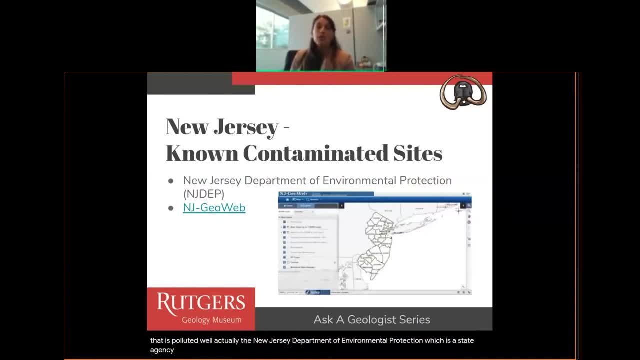 Environmental Protection, which is a state agency whose mission is to protect the environment and human health, has compiled a statewide database that contains all known contaminated sites in New Jersey, And anyone you know- you, I, anyone- can access this website- type in an address to see if there are any contaminated sites near you. So just to show. 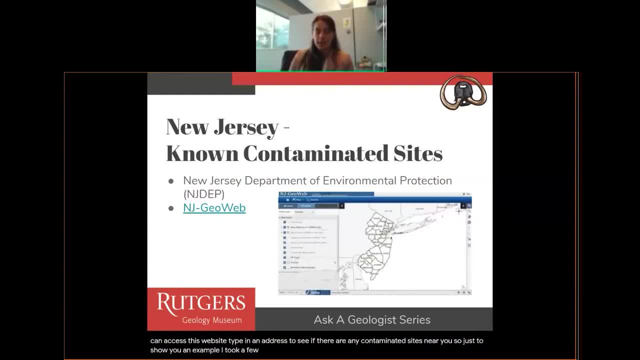 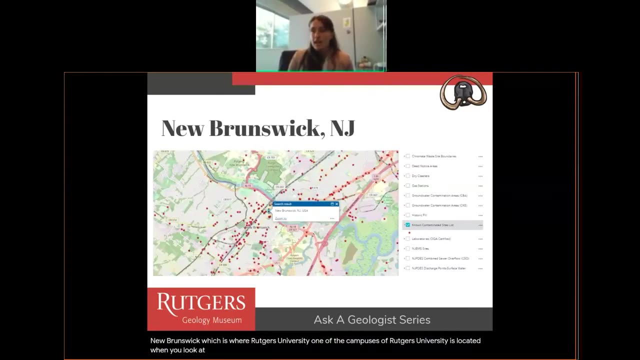 you an example. I took a few screenshots from the website of different locations. So first let's look at New Brunswick, which is where Rutgers University, one of the campuses of Rutgers University, is located. So when you look at this database and you check this layer called known contaminated sites, little stars will appear wherever there's. 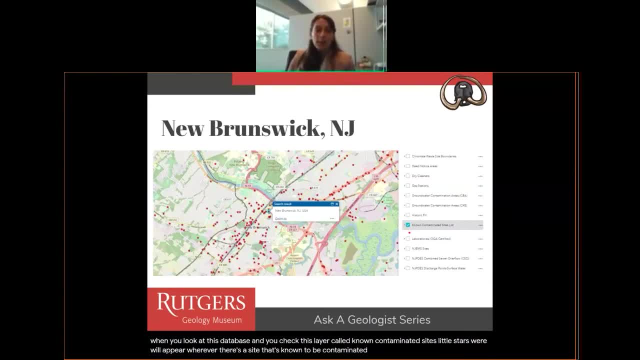 a site that's known to be contaminated, And you can probably see that. you notice that there are more red stars right at the center of the city of where New Brunswick is, And that's because there are a lot of people there, And it's also important to note that cities are built usually near water. 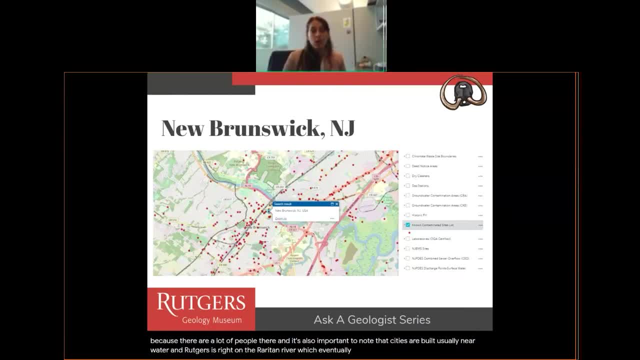 And Rutgers is right on the Raritan River, which eventually runs into the ocean, And surface and groundwater that flows into the Raritan River can pick up a lot of contamination from cities and bring them into the ocean. All right, let's go. 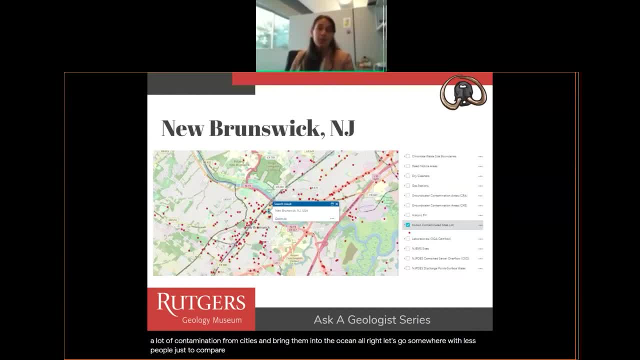 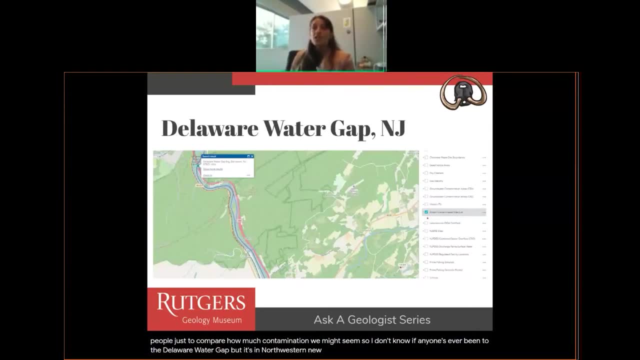 somewhere with less people, just to compare how much contamination we might see. So I don't know if anyone's ever been to the Delaware Water Gap, but it's in northwestern New Jersey and it's a national park. So I typed in Delaware Water Gap into that into GeoWeb, and I could really not. 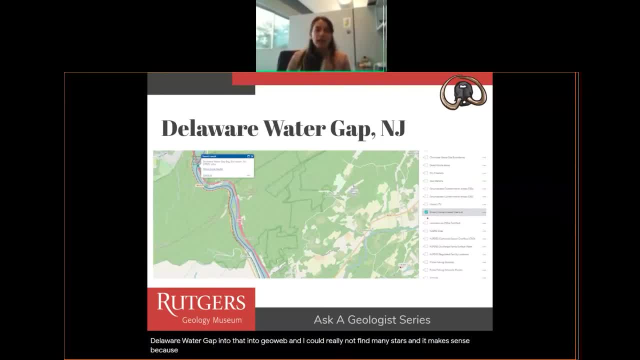 find many stars And it makes sense because preserved land and people can't live there And often there's a lot of known contamination where people are living. So in this particular location I only saw one little star as I was moving around in this area, So you can see there's. 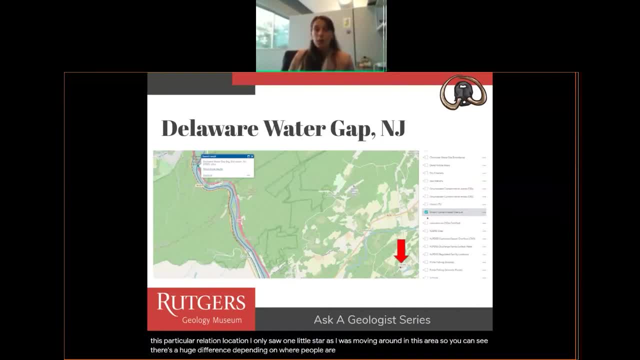 a huge difference depending on where people are. And one more example: let's now go somewhere. Let's go to a very dense city where there are a lot of people and factories and industries, like Newark, New Jersey. So Newark, New Jersey. as I just said, it's a very dense city and there are a lot of industries there, And so there are a lot of stars, and it's right there next to a water body. So go ahead after this if you want and look. 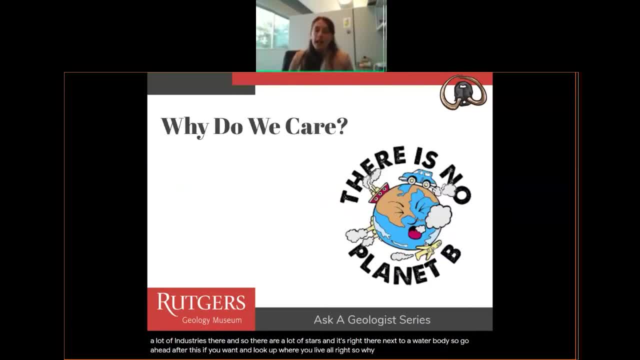 up where you live, All right. so why should we care, right? So, first of all, we only have one Earth right, And Earth is indescribably unique and it's our home. We're adapted to survive on. 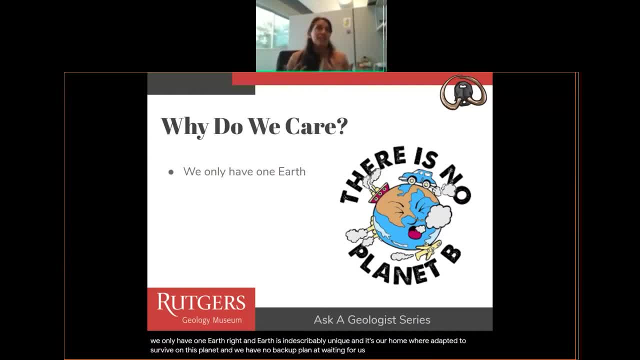 this planet and we have no backup planet waiting for us. So we have to survive on this planet and we have no backup planet waiting for us that we can live as comfortably on as we do on Earth. So we have to be mindful of how we treat our planet, especially if we want our children and 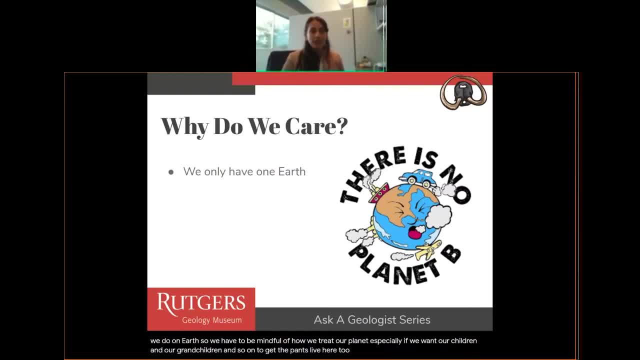 our grandchildren and so on, to get the chance to live here too. Let's see why else. Oops, Okay, sorry, too many, All right, so another thing is that when people and animals and plants are exposed to polluted air, water or soil, there are a lot of negative 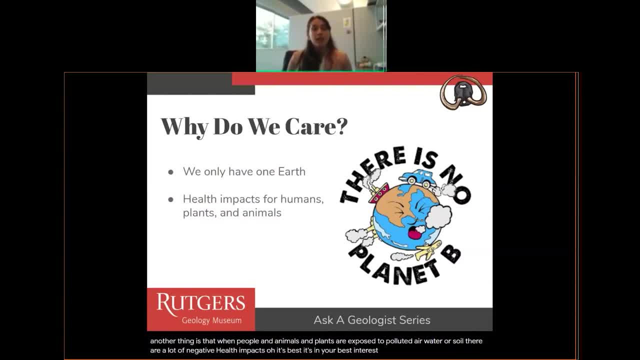 health impacts, So it's best, it's in your best interest to care so that you stay healthy. Air pollution impacts our respiratory systems and we need healthy respiratory systems to combat respiratory illnesses like coronavirus, which are becoming more commonplace. And the last reason is- I'm sure you know, you've likely heard about 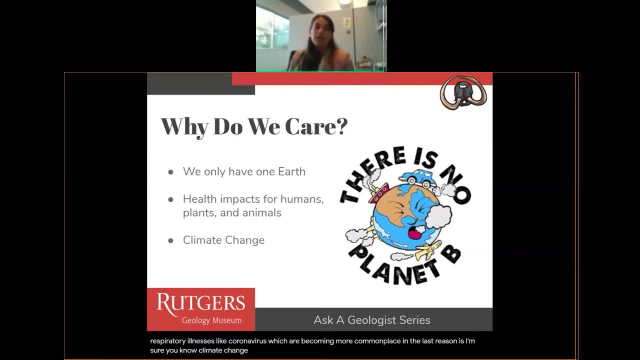 and that's climate change. Climate change is directly linked to pollution, specifically man-made pollutants such as greenhouse gases that are emitted into the air. So if you're in a desert, you're going to have a lot of air pollution. So if you're in a desert, you're going to 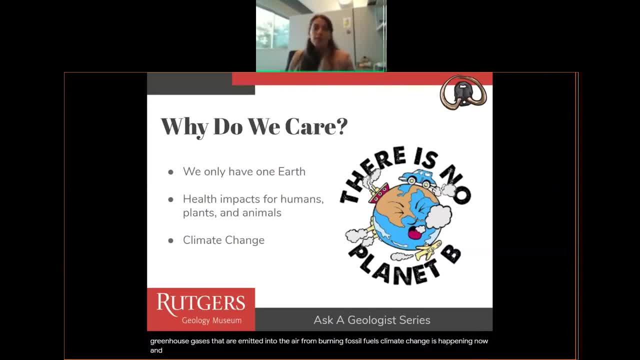 have a lot of air pollution. So if you're in a desert, you're going to have a lot of air pollution. Climate change is happening now and our Earth's equilibrium is shifting. temperatures are rising, sea levels rising. There are so many other consequences of climate change that are 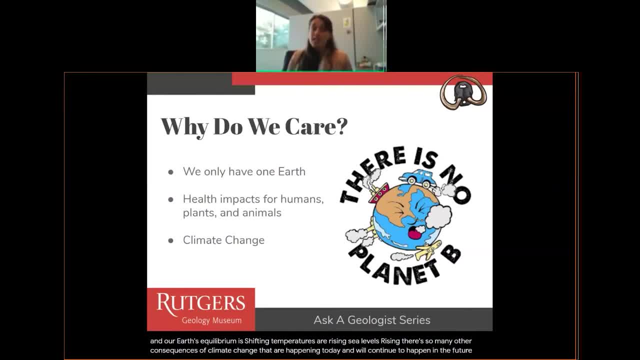 happening today and will continue to happen in the future. And, as young individuals, it's in your best interest to care about these issues, because, while it might have been your parents or their parents who have contributed to climate change so far, you will be the one who has to adapt to. 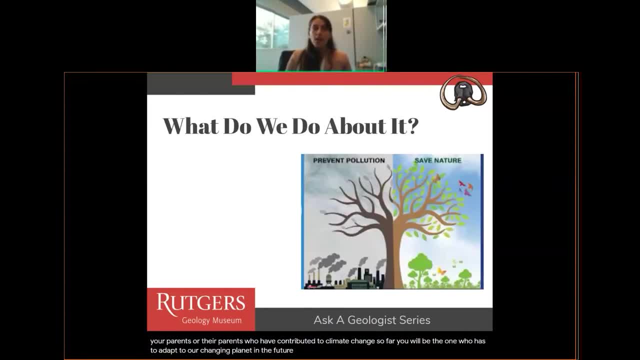 our changing planet in the future. All right, so what can we as a human population do about it? to prevent pollution, right? So at the governmental level, laws can be passed that will protect the environment and human health. The EPA, which is the Environmental Protection Agency, is an executive agency of. 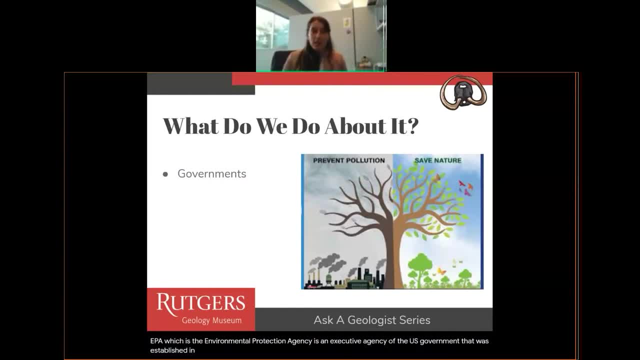 the US government that was established in 1970, and it manages environmental protection matters. Businesses also need to be held accountable For their actions. a business-as-usual attitude is no longer acceptable. They need to implement sustainable practices and find ways to be successful. 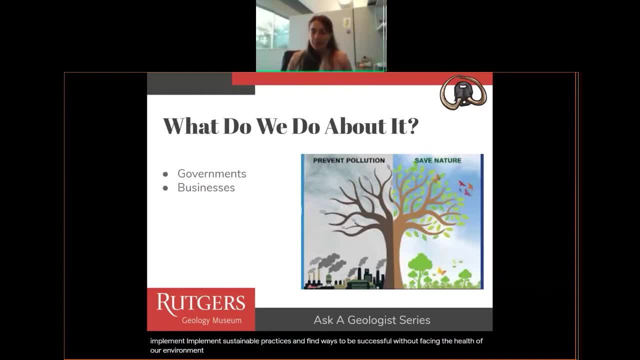 without sacrificing the health of our environment. There are a lot of environmental groups, like the Sierra Club, which seek to protect and monitor the environment. They spread awareness, they hold people and organizations accountable for their actions and they push for change. So the EPA is up to date on all of the measures they see to tryin'. 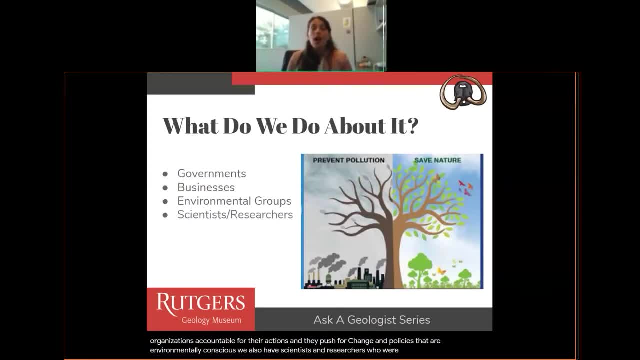 to protect people from a natural character, by education, by social justice and by environmental consciousness. We also have scientists and researchers who work on understanding the impacts of contamination, And they also use technology and their knowledge to come up with ways to clean up the environment. 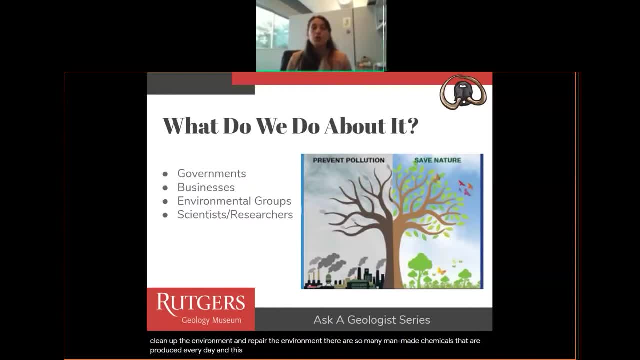 and repair the environment. There are so many manmade chemicals that are produced every day- and this list continues to grow- emanates that appear all the time that we're still learning about their impact, So it's a very important role that scientists and researchers have too. There are also educators who play a 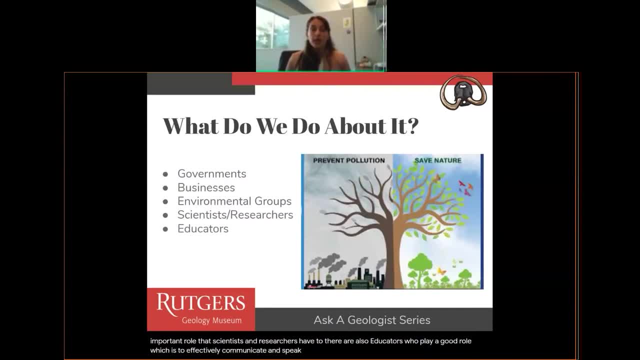 good role, which is to effectively communicate and spread the word, and like we're doing right now and you also have the opportunity to do. And then, at the individual level, there are many things that you can do to play a part, and I will discuss more specifically in a little bit, But for now, 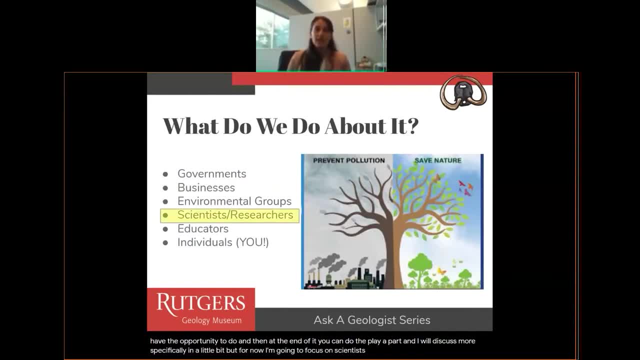 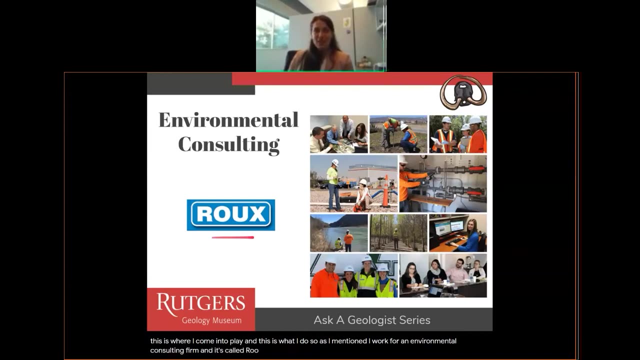 I'm going to focus on scientists, researchers, because, as a geologist, this is where I come into play and this is what I do. So, as I mentioned, I work for an environmental consulting firm and it's called Roo, which you can see here. So environmental consultants consist of geologists like myself. 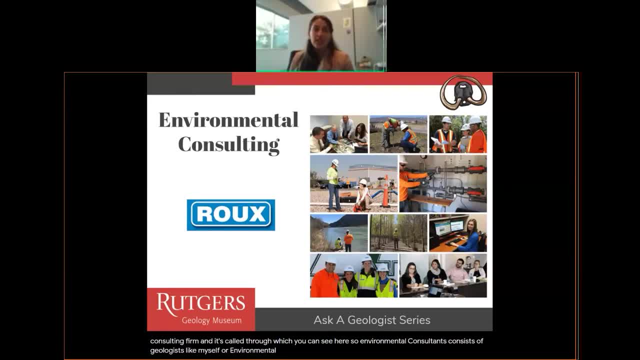 or environmental scientists or engineers, and we use our expertise and our knowledge in our field to to advise businesses and governmental agencies on the best practices for cleaning up contaminated sites and preventing future contamination. So we try to solve some of the most challenging and complex environmental problems and find sustainable solutions, And me in particular, my job. 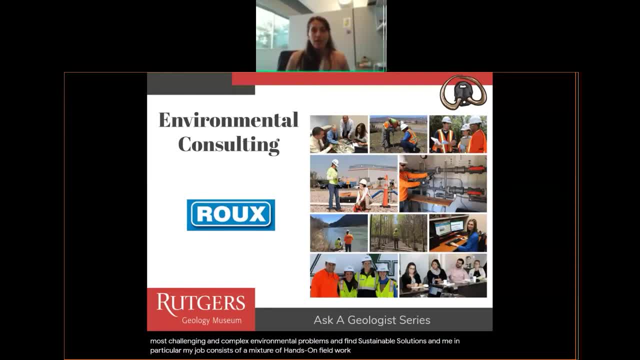 consists of a mixture of hands-on field work and office work, And before we can come up with a solution to remediating or cleaning up a site, we first need to assess the state of contamination, And we can often achieve this by sampling the soil. 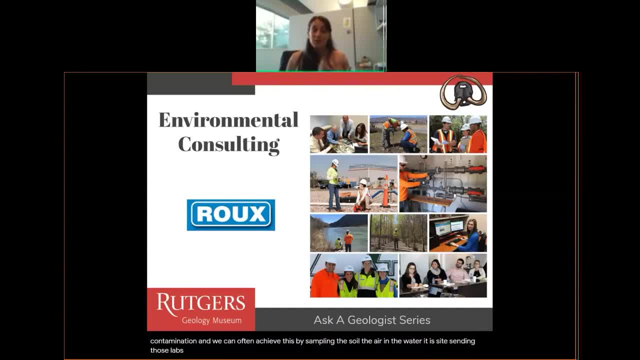 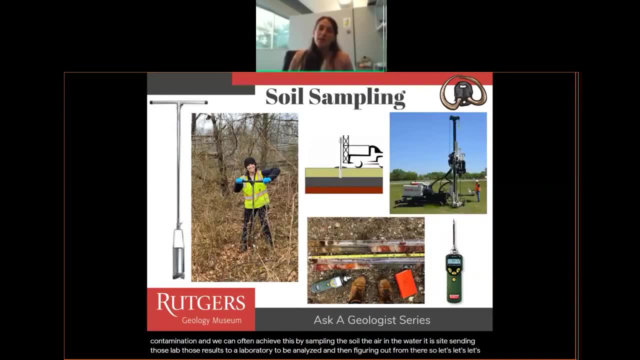 the air and the water at a site, sending those lab, those results to a laboratory to be analyzed and then figuring it out from there. So let's, let's, let's talk about soil sampling a little bit. So we can collect soil samples many different ways. One way is you can use a hand auger, which 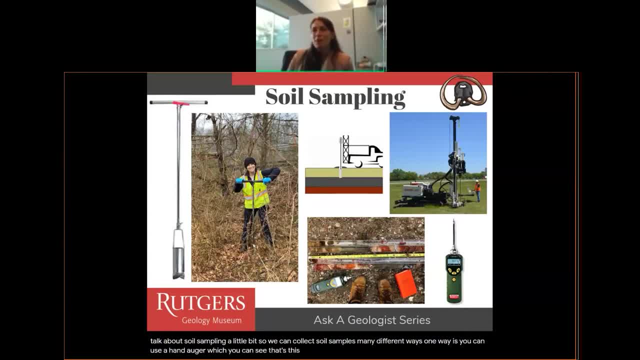 you can see that's this instrument, this piece of equipment that I'm using here, where you twist it and push it into the ground and you're able to pull soil up. But hand augers can only retrieve soil at shallow depths like. this is maybe a five feet, So if you need to collect soil much deeper, 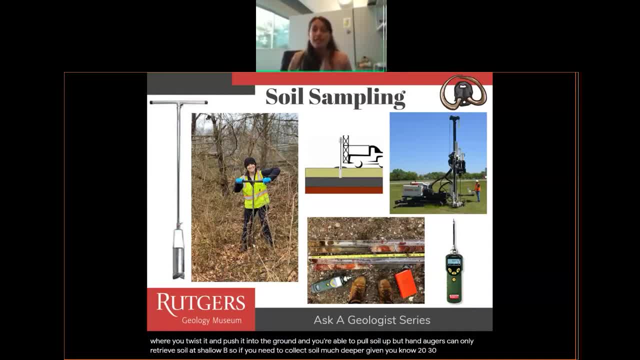 even, you know, 20,, 30,, 40,, 50 feet deeper. you can install soil borings, And a soil boring is essentially like a giant straw that you stick into the ground, and when you pull that big straw up, you get a lot of soil. 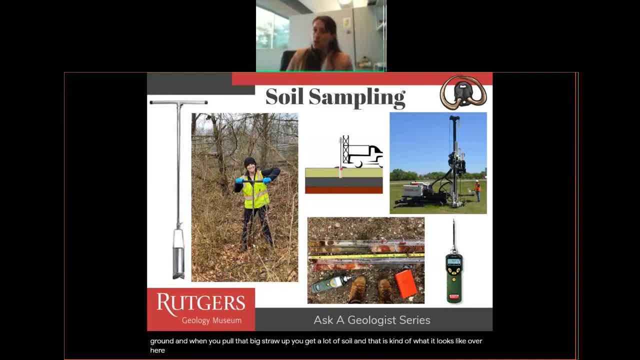 And that is kind of what it looks like over here: like a big straw you stick into the ground And when you pull it up it'll look something like this: And in order to push that straw into the ground you need a lot of force. 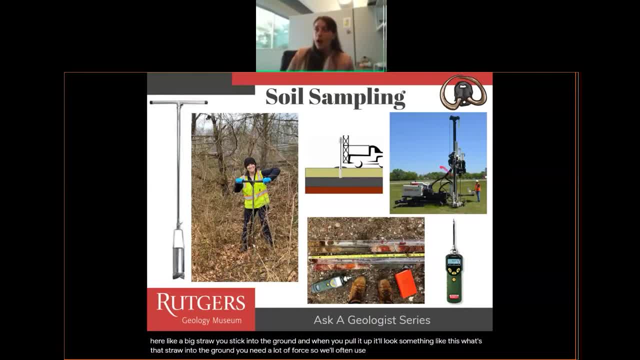 So we'll often use a drill rig, or we'll hire someone to operate this drill rig and push down to the depth that we want them to in order to retrieve this boring log. And in the boring there's a lot of soil and over the云you can see here there's a lot of sand, there's a lot of clay, There's a lot of moss. 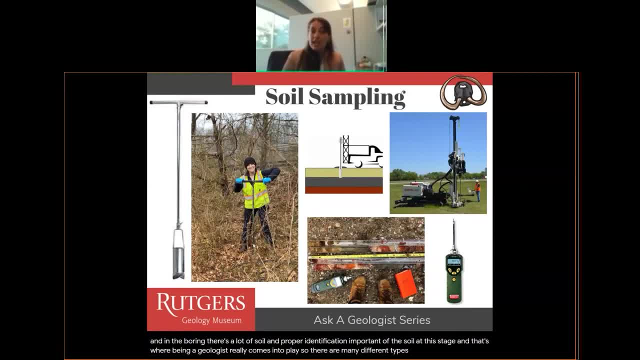 there's a lot of pebbles, there's a lot of sludge, So there's a lot of soil. I think another important part of soil identification is a very important of the soil at this stage, And that's where being a geologist really comes into play. So there are many different types of soil, like sand, silt, clay, cobbles, and then there are just rocks as well that you need to think about too, And each contamination will behave differently in each different type of texture. So, for example, you could imagine 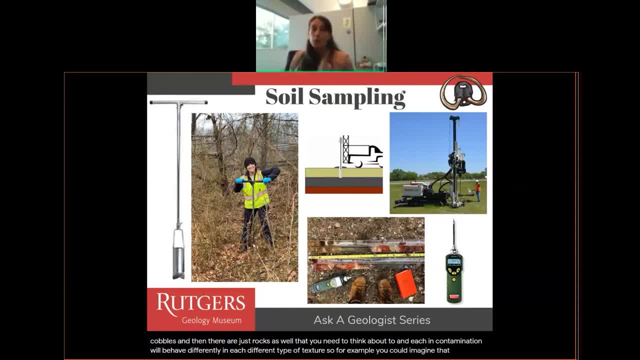 that contamination would travel really quickly through a layer of sand, since it's very loose and there's a lot of space between the particles. once you reach a clay, where there's less space between the particles, the contamination might stop, and this is important so we can predict the behavior of 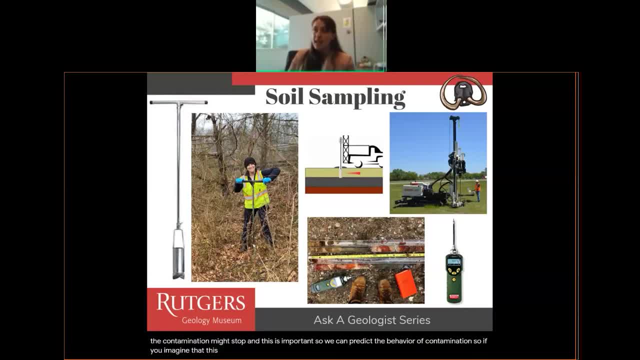 contamination. so if you imagine that this tannish layer is sand and contamination and some oil was spilled right, it might travel down into the sand and stop once it reaches this dark layer. maybe it's a clay, and so by characterizing and understanding soil you can really predict where. 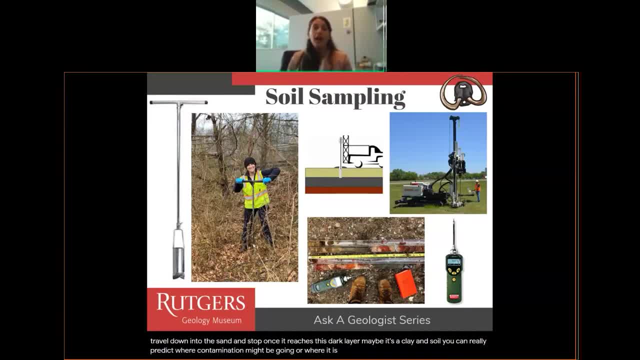 contamination might be going or where it is, and find a way, a solution, to clean it up, and one of the ways in the fields, when we look at the soil, that we can identify if it might be contaminated, other than collecting a sample and sending it to a lab to be utilized, is you can use this instrument and it's. 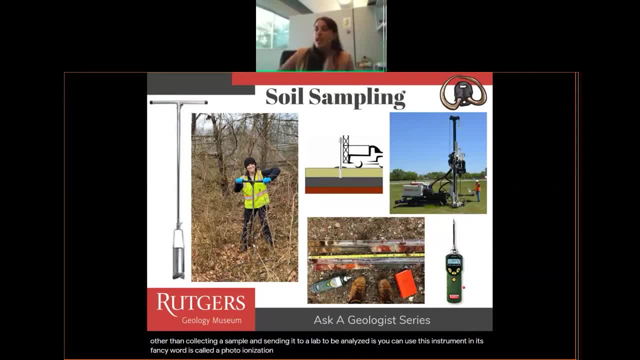 fancy word. it's called a photovoltaic photoionization detector and it's basically like a sniffer that can sniff out if there's contamination, and you hold it up to the soil and you can scan it, figure out where the contamination is. all right, so there's also groundwater. 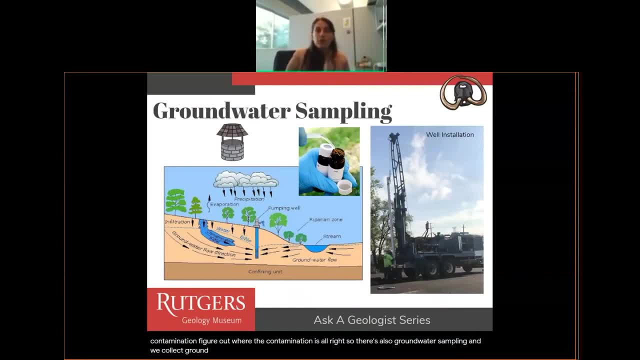 sampling and we collect groundwater samples from a well, which also is like a big straw or like a tube that goes into the ground, and the photo on the right here shows another drill rig that is actually installing a well into the ground and that's that big. it really does look like a giant straw and they're gonna. 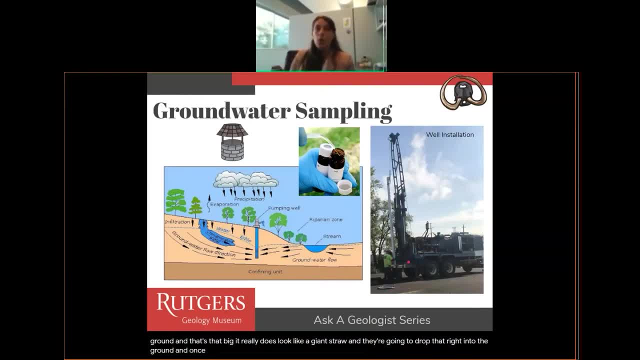 drop that right into the ground and once it's in the ground the water will flow up into the tube and then we can pump water from the well into our sample. so you can kind of imagine just how important understanding water contamination is. imagine that this is, this is a well, right here and people 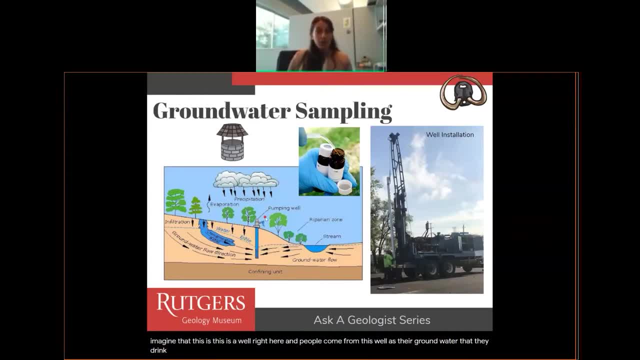 pump from this well as their ground water, that they drink from it like a drinking well and someone spilled some sort of a chemical up here. you'll get this. it's called a plume, which is an area of groundwater that's contaminated and that groundwater while you spilt something over here or someone spilt. 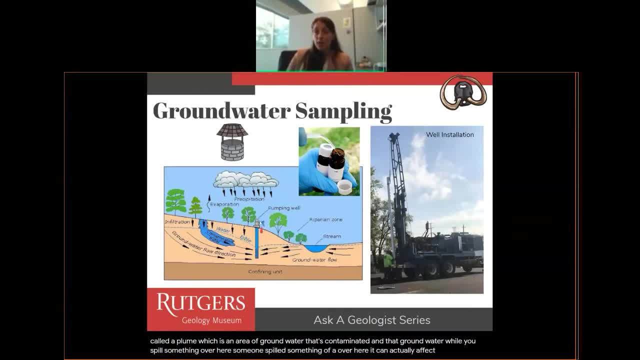 something over here, it can actually affect this person's drinking water down here, as the water can move underground and, once again, when you understand the layers of soil and the geology that the water is moving through, you can predict where the water might be going and who might be receiving that contamination. 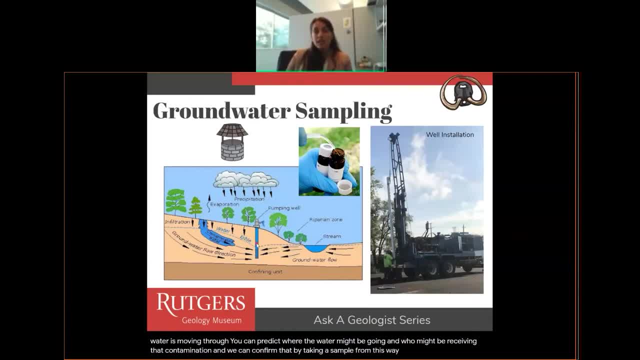 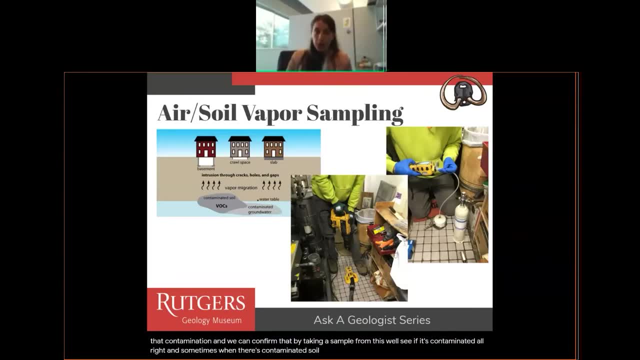 and we can confirm that by taking a sample from this. well, see, if it's contaminated, all right. and sometimes, when there's contaminated soil, soil or groundwater, vapors can fill the spore, the pore spaces- remember how there was air in between the soil particles? and it can. the vapors can fill those spaces and 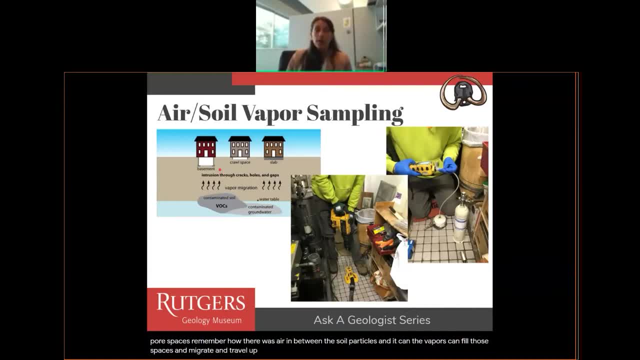 migrate and travel upward toward the surface of the earth, and then it can move up towards the surface of the earth, and then it can move up toward the surface of the earth, like this figure shows here, and the soil gases can actually migrate through cracks in your basement crawl spaces and 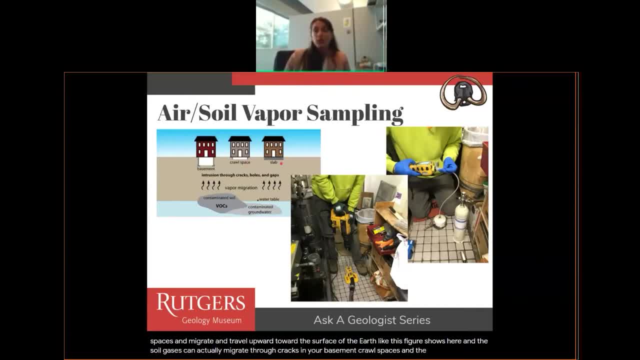 the foundation of your home and actually seep into your living space. and I know a lot of times in New Jersey radon, which is a natural gas- I mean it's it, it naturally occurs right- can often seep out of the bedrock and into people's. 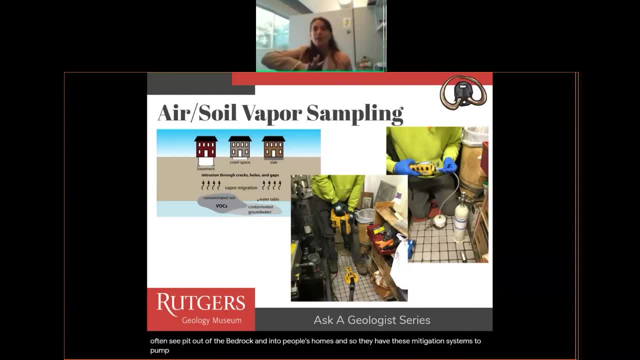 homes and so they have these mitigation systems to pump that air, that radon from underground out of their house so it won't be into their homes. and similarly, when you have contaminated soil or groundwater, like for example if you had a gasoline spill, those vapors actually are volatile, they're called volatile organic carbons. 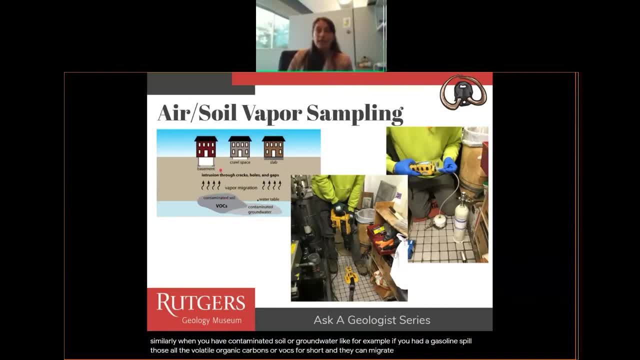 or vocs for short, and they can migrate upwards and get into the cracks of your house. so what we do is we can sample both the ambient air that you're breathing in your basement, for example, or the first floor of your house to see if any of those contaminants are in the air, and we can also, as a 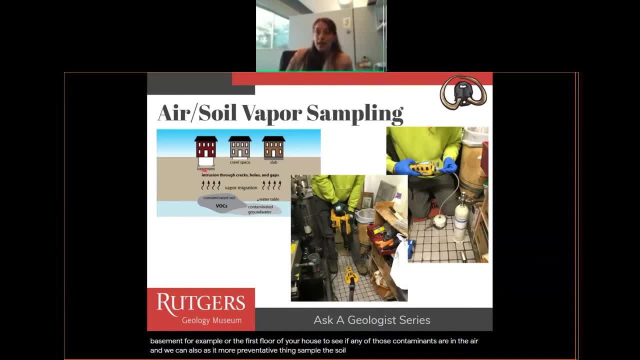 more preventative thing: sample the soil, air, the air in between the pore spaces of the soil underneath your house, to figure out if there are contaminants that could seep and migrate into your house. so the way that we would do this is we drill a hole through the floor of your house, right, right. 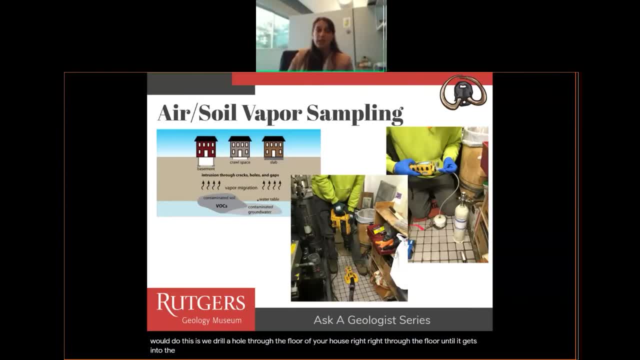 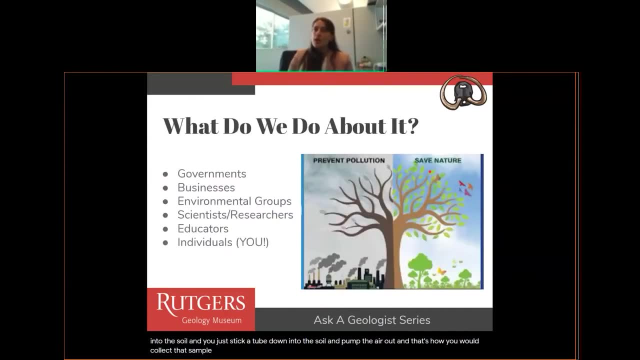 through the floor until it gets into the soil and you just stick a tube down into the soil and pump the air out, and that's how you would collect that sample. all right, so you know I talked a lot about what I do to prevent pollution and to clean up pollution. 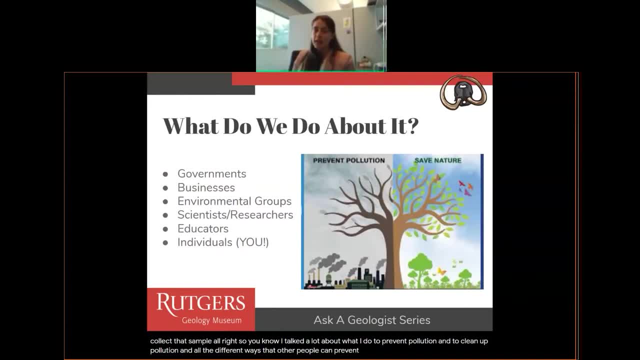 and all the different ways that other people can prevent pollution, but I just want to, before I end, talk a little bit about what you can do. so, first of all, you have the power to educate your friends, your family, parents, your teachers, anyone, um, for anyone who wants to listen to what all the узra is saying, to um. 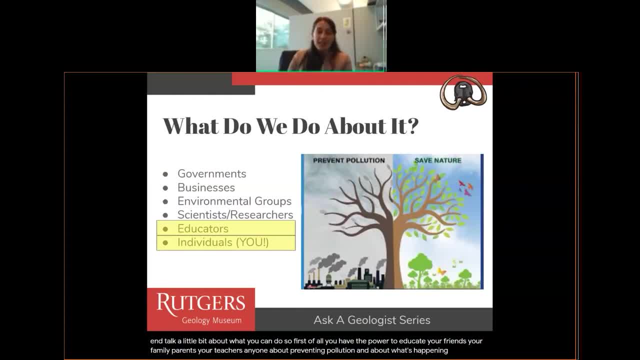 your family. you can go back and listen to what you can just plug on a device. plug on a device, check it open, send a message to the teacher. you know, give that message to someone. go and ask if they have COVID um The Cao um person in the room right now there, like the nurse said. you know, if you knew about it I'd send a note to your повтор. 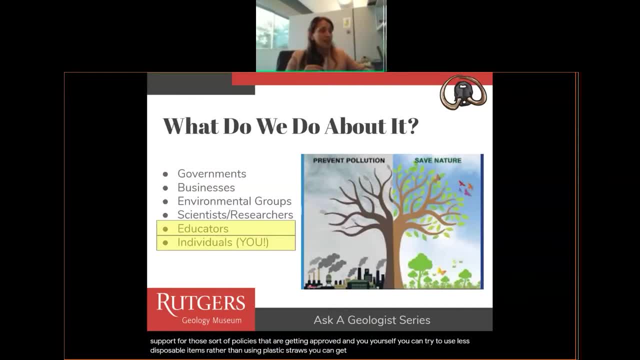 You will understand, rather than using plastic straws, you can get like a, like a reusable straw or um. you can bring your bags with you when you go to the store. you can even pick up items and recycle them if you see them on the ground. i'm sure your parents remind you to turn off your lights and your electronics. 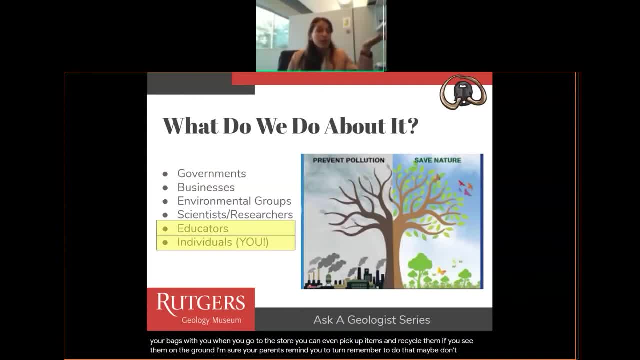 you can always remember to do that. maybe don't run your water too long when you're rushing your your, when you're brushing your teeth? um, use refillable water bottles. figure out, you know, can you buy less? are there things you can buy that are reused? um, maybe you can tell your. 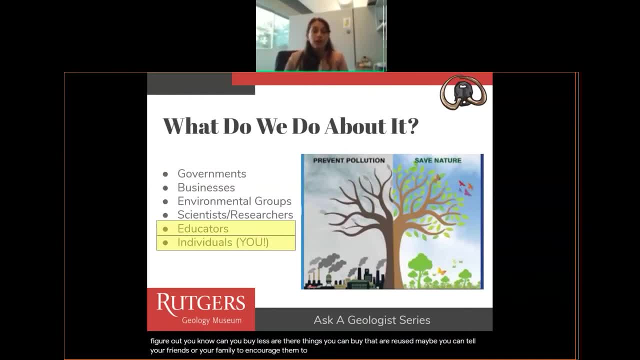 friends or your family to encourage them to buy food and clothes that are made without pesticides? um, yeah, there are a whole list of things and if you're interested, um you know, you can always reach out, because there are definitely. even though it feels small, it makes an impact. 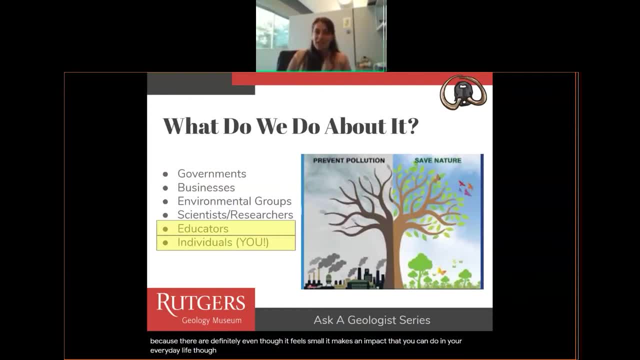 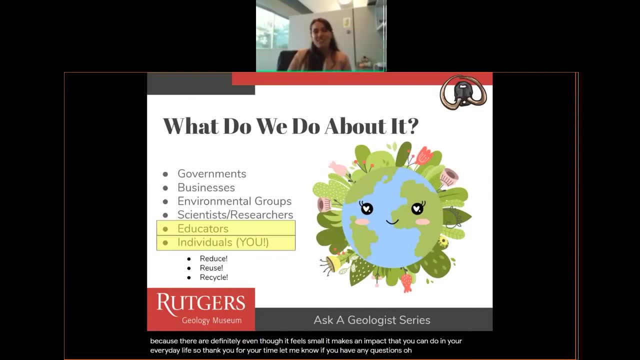 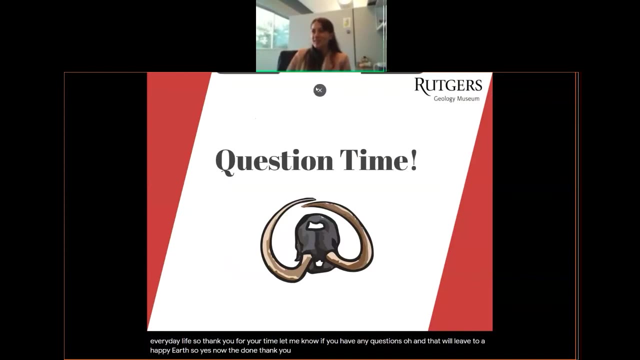 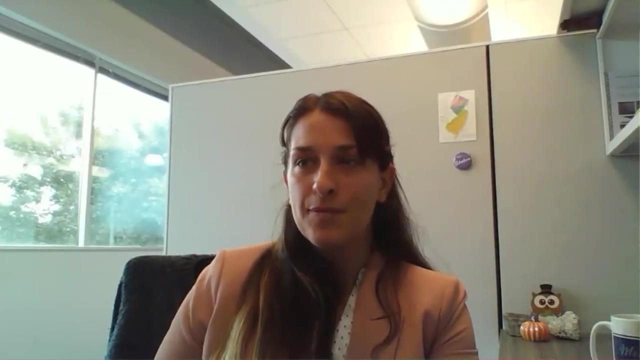 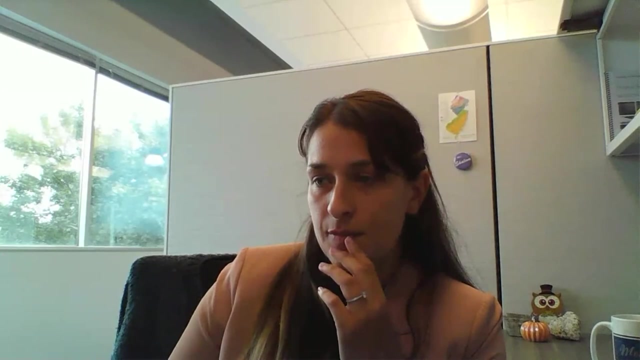 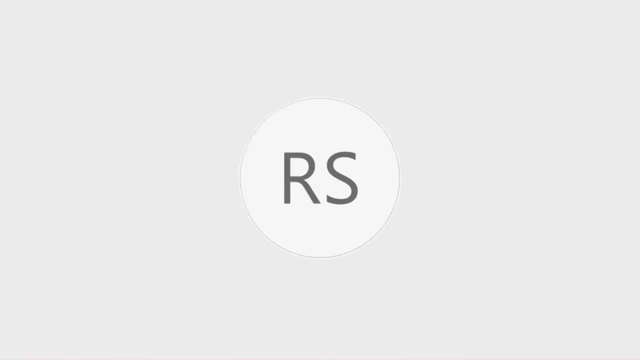 that you can do in your everyday life. so thank you for your time. let me know if you have any questions. oh, and that will lead to a happier. so yes, now I'm done. thank you, okay, Monica, you can go ahead and answer the questions, all right? okay, let's see. all right. 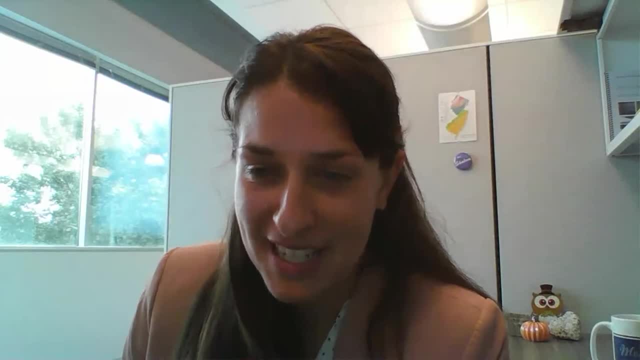 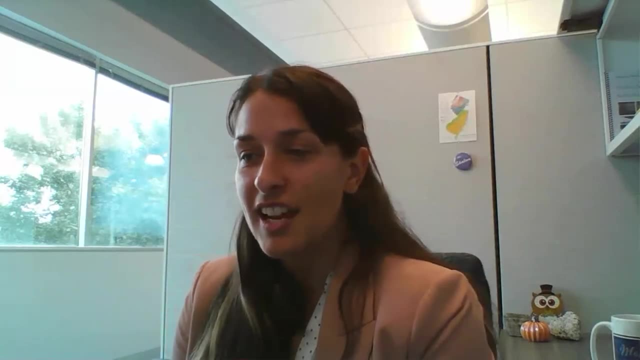 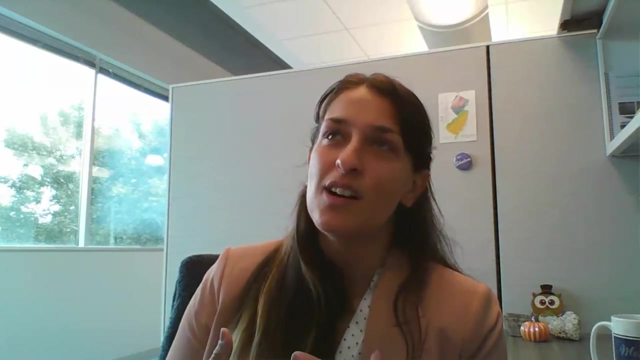 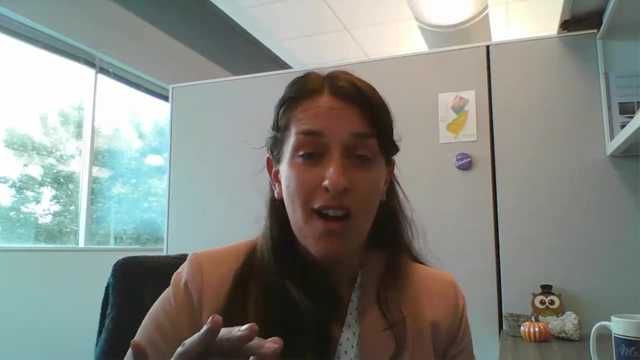 well in the chat I see one from my dad. actually, how much time do we have to stop climate change? that's a very good question and I think it's really debated. and stop climate change. it's kind of may be difficult to just stop it, but because even right now, if we were to stop all of 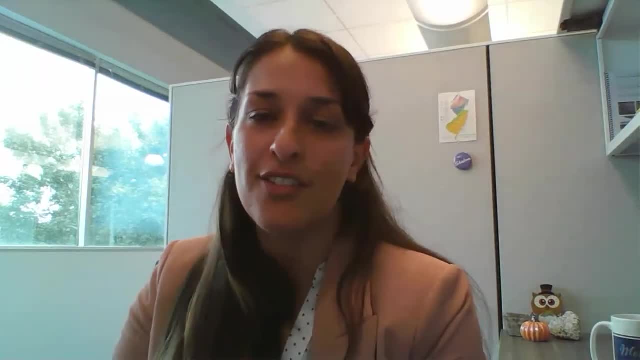 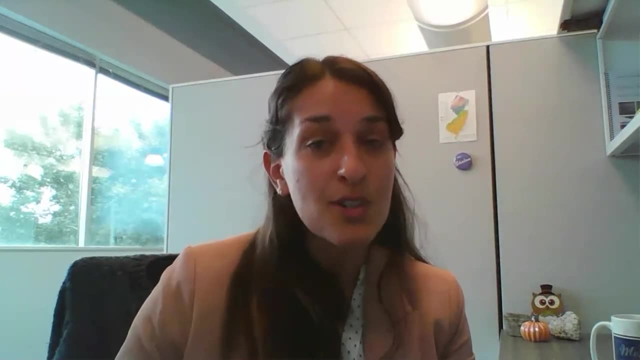 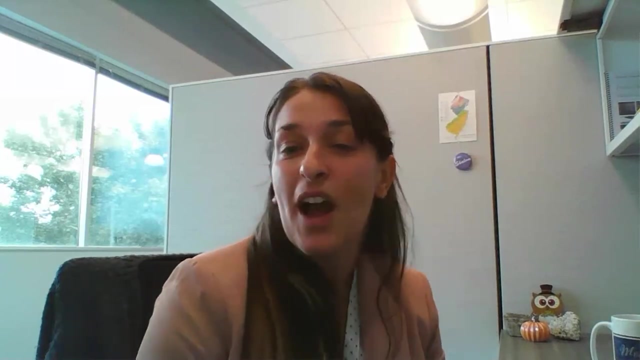 our emissions of greenhouse gases and stop burning fossil fuels. there's a lag, there's like a delay, and impact on the earth and temperatures are would still rise even if we stopped everything today. but that doesn't mean you shouldn't try, because obviously if we continue as business, 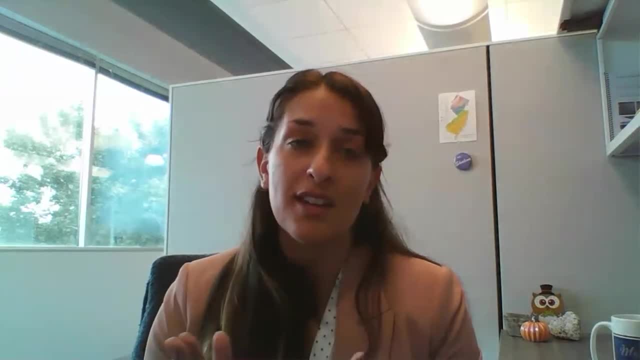 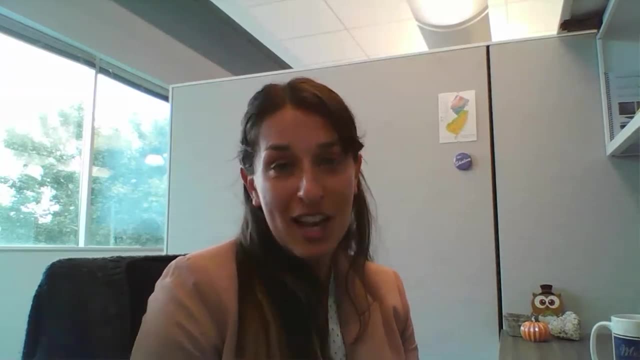 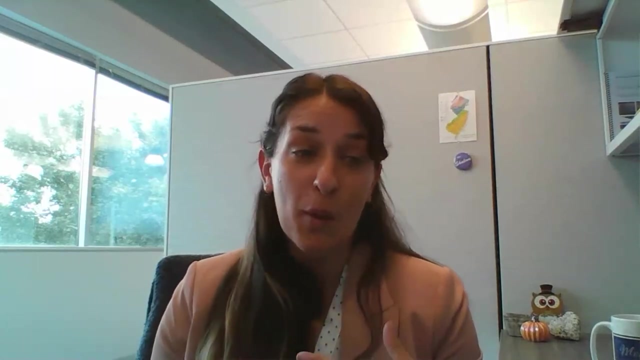 as usual, temperatures will rise a lot more than we're really prepared to handle. so I know there's actually I was talking with Rhea about this yesterday. there is a clock in Times Square that's called, like, the climate change clock or something, and if you know more about 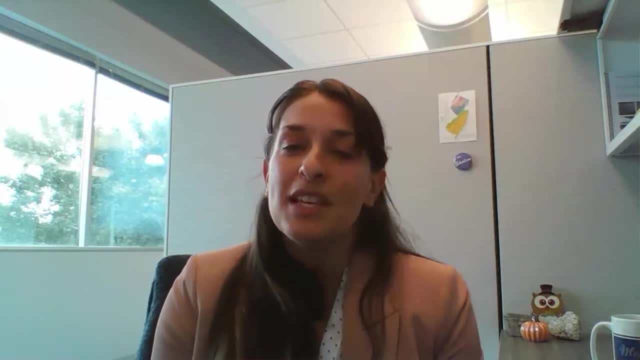 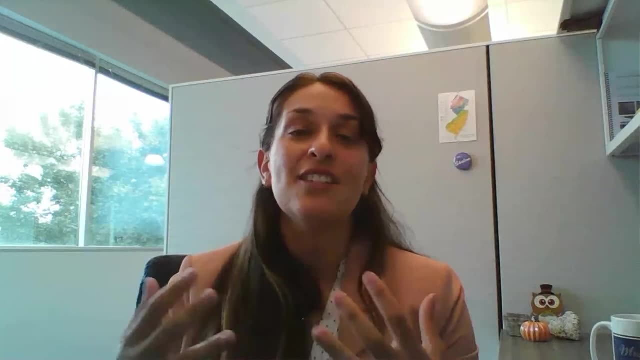 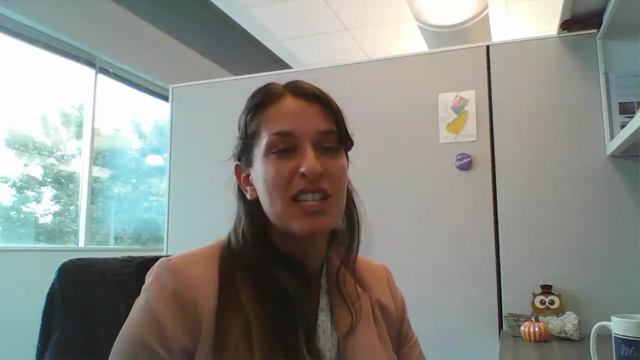 it, let me know, but this clock is putting seven years until the amount of it gives us basically seven years, until the amount of impact that we're going to be causing will be too much for us to handle. so and that, essentially, is being calculated by you know, we have seven. 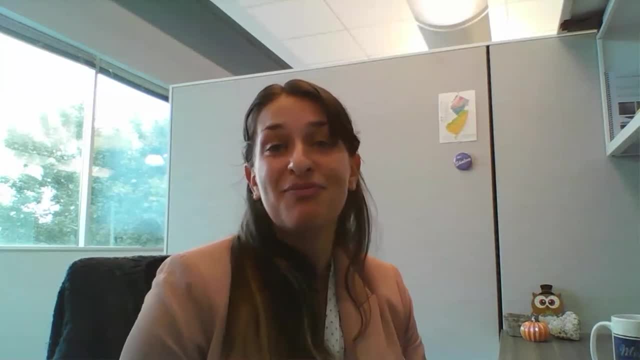 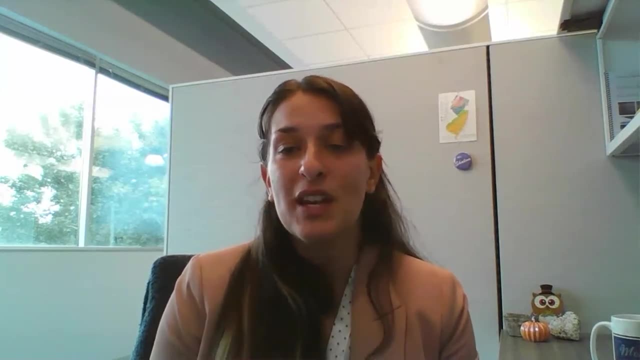 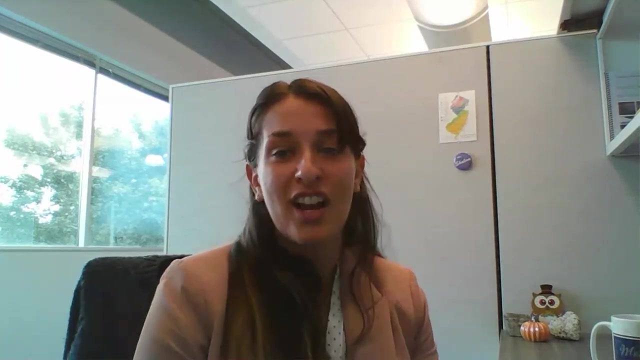 years to do something until it's really too late to you reverse or, you know, repair the for us to live comfortably. So it's a good question, and I think that, rather than asking how much time we have, we should just start now trying. Okay, let's. 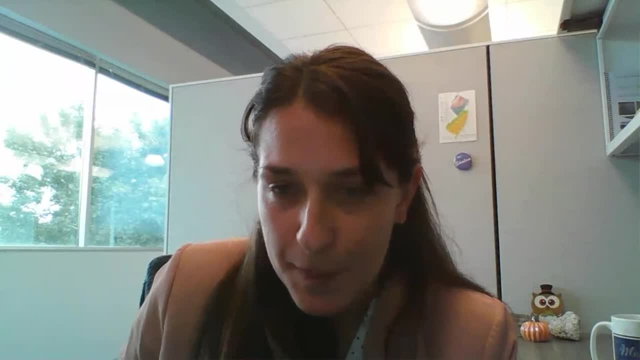 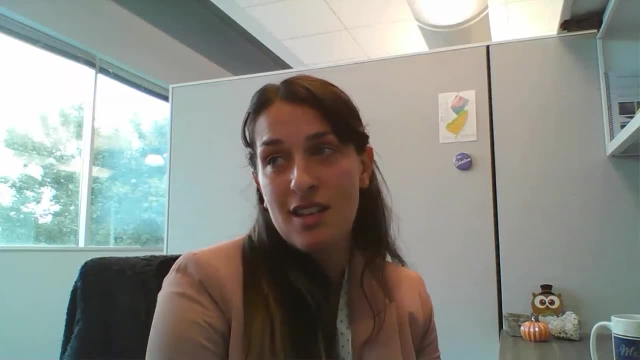 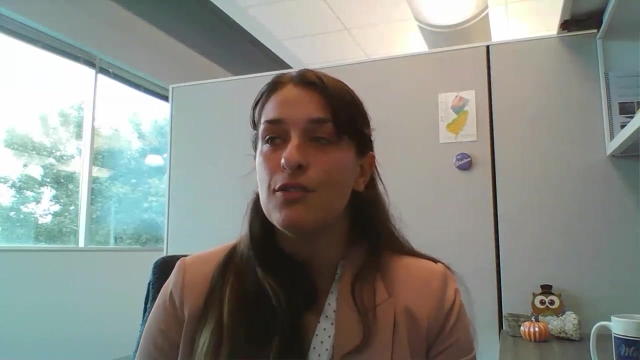 see what else there is All right. so is pollution generated more from humans or from natural causes? So that's a good question. if I were to guess, I would say from humans, and in fact it's kind of related. So you've been hearing probably. 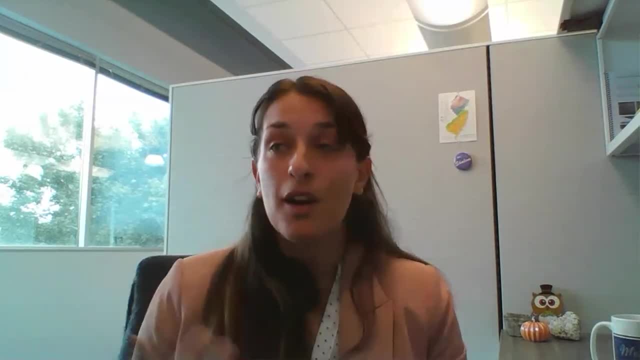 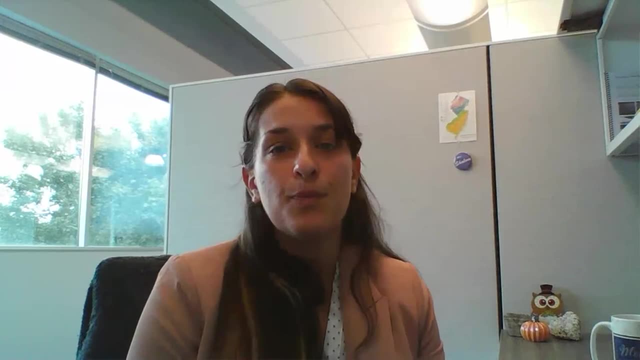 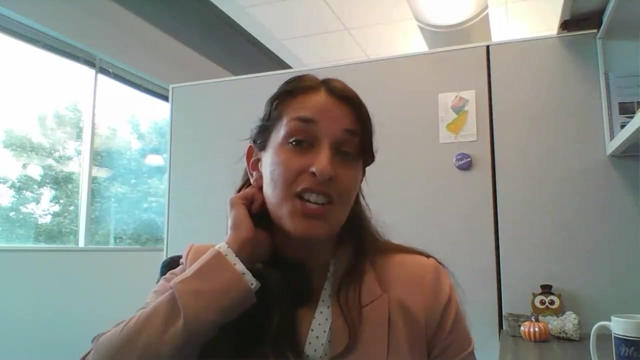 about these wildfires that have been happening all different parts of the world. and while wildfires are a natural phenomenon that take place, climate change- and you know, which is, you know, caused by emitting fossil fuels- can actually exasperate the impacts of wildfires, and so the two can be. 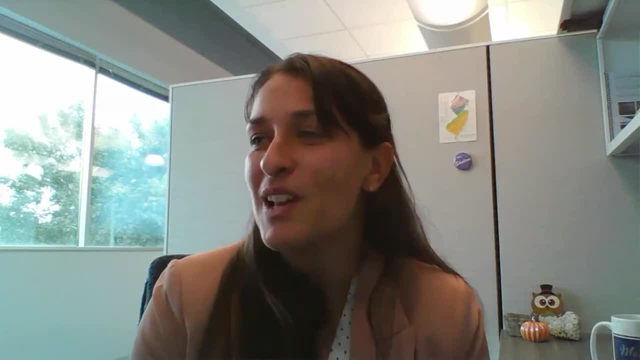 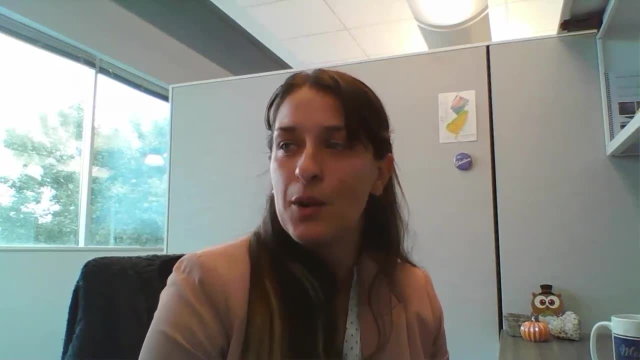 pretty related. Have there ever been any oil spills in New Jersey? That's a good question. I'm not sure if there are any big or notable ones, but small oil spills for sure. Most gas stations I've seen have had some sort of an oil spill. but one of those huge oil spills like the BP oil spill- I haven't heard about that, but I don't know. Let's see: How did the drinking water in Newark, New Jersey, get contaminated with lead? I'm pretty sure that that was actually from partially from rusting pipes which are made. 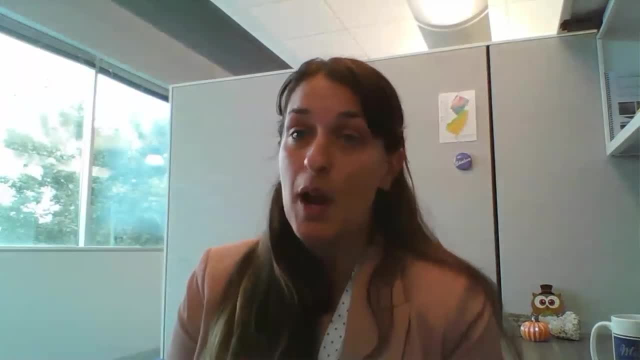 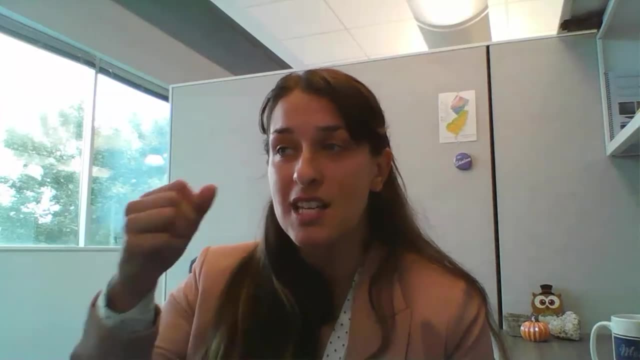 with lead can go into the groundwater when they're old and not repaired, And I remember one time I was sampling water in a school in Newark and we opened up the faucet and the water that came out was yellow, which was really gross. 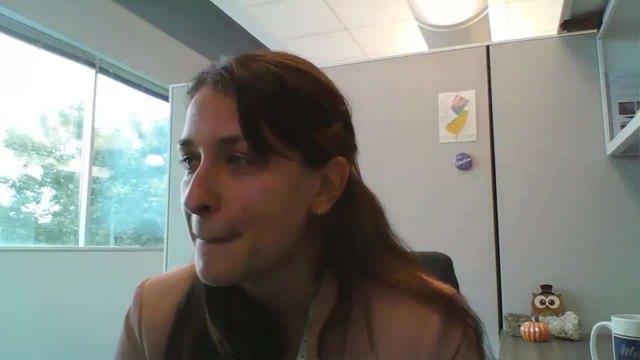 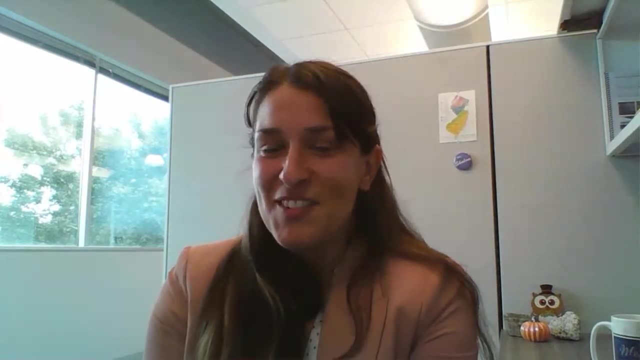 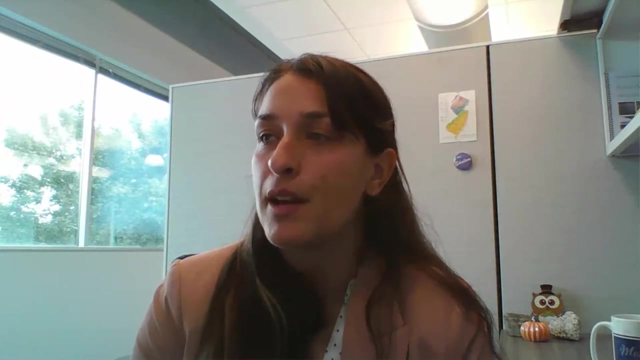 Okay, All right, Ria's mom would like to know. thank you, Ria, for Ria's mom for listening today. Recently, many beaches on Long Beach Island, LBI, have been closed because of bacteria in the water. For example, Surf City has had a lot of bacteria and I want to know where did 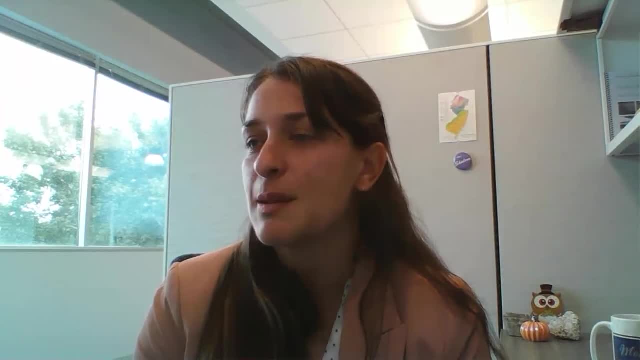 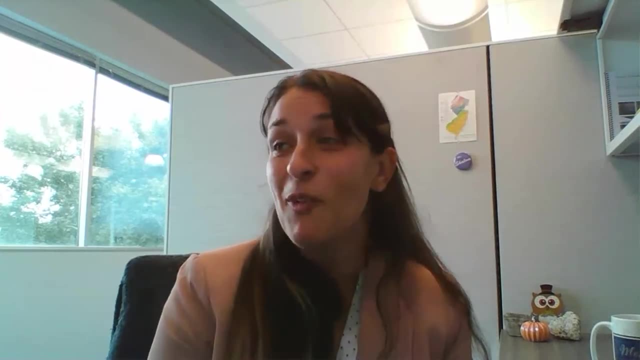 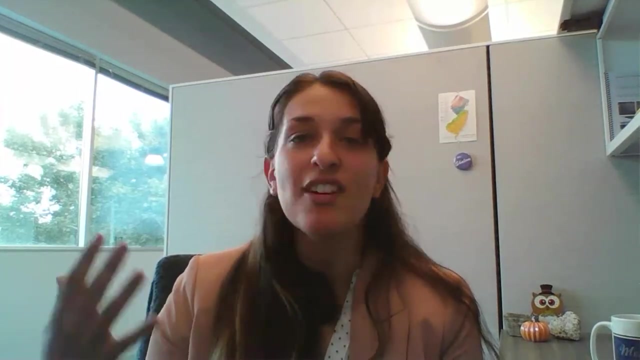 that come from? Does it have anything to do with older, rusty pipes? That's a very good question And I can't tell you with certainty where exactly the bacteria comes from. But just from you know this presentation, you can see that everything. 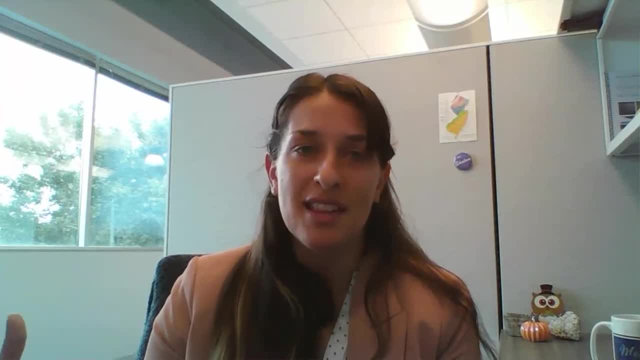 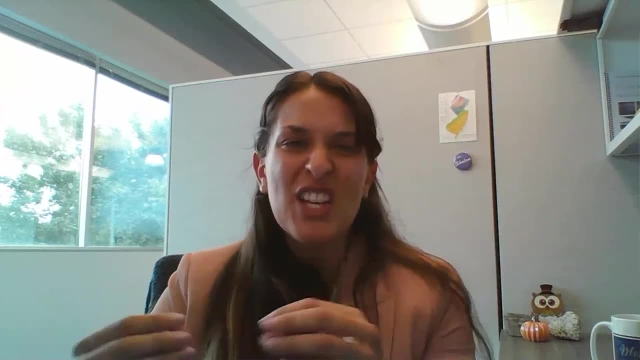 drains to the ocean And and there are so many ways that all these nutrients and all these other- you know- fertilizers and oil and all these things that get washed off the land and into the ocean can really negatively impact the ocean, But specifically the 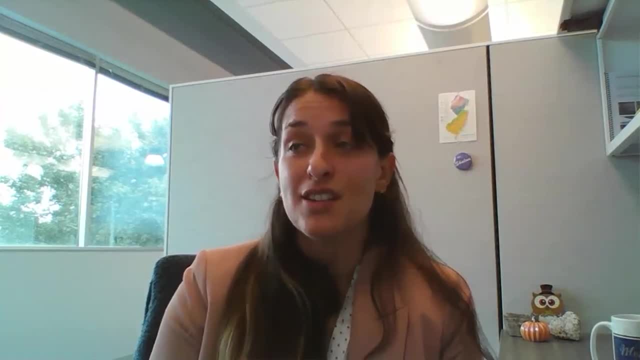 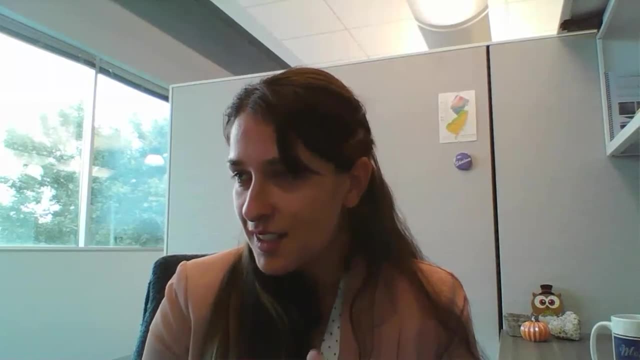 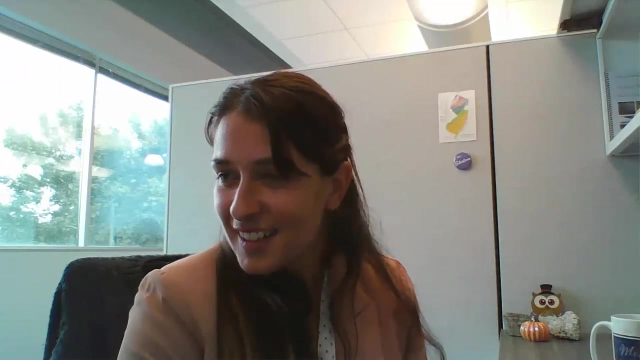 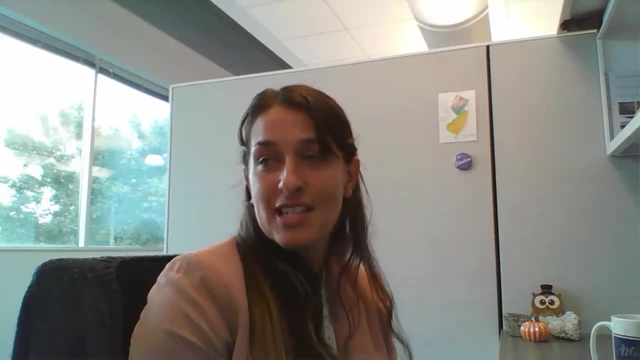 bacteria. I don't know exactly where that comes from. I'm interested to find out, though. All right, Let's see. Okay, Okay, so how is pollution linked to the loss of species here in New Jersey, from Mary in Scotch Plains? So? 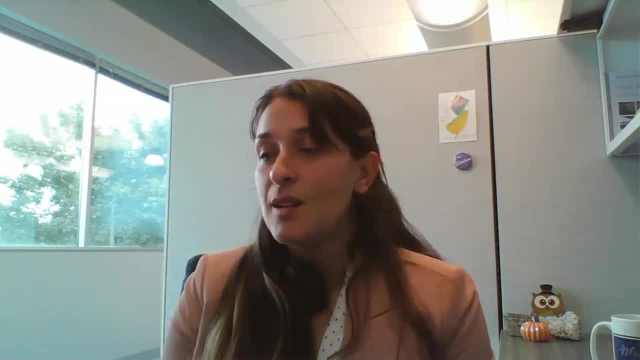 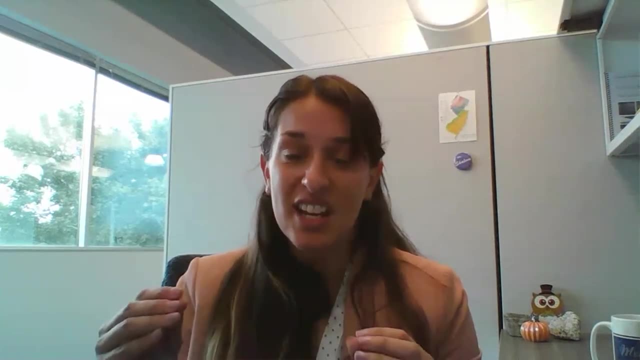 You might have noticed um plastic. you probably have seen like pictures of fish and marine life getting stuck in plastic and eat, ingesting and eating a lot of plastic and, for example, in new jersey's pacific. 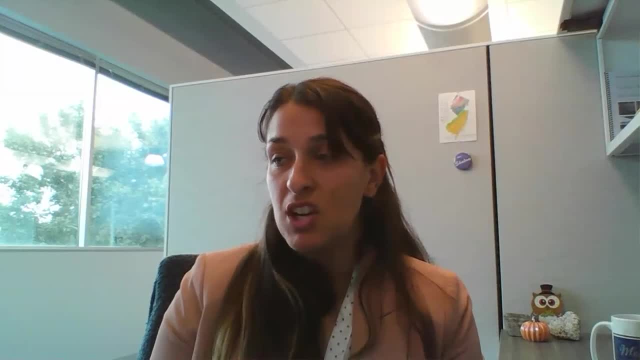 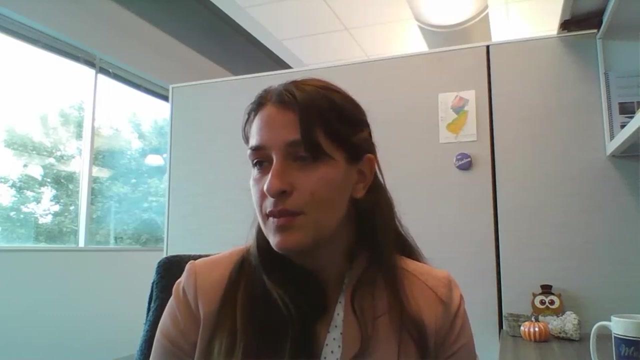 example? um is that ospreys actually collect a lot of trash and use them as nesting material, and it can sometimes entangle them and trap them and kill them. um, let's see what else we can do with this. what is the most difficult pollution to undo in the environment? 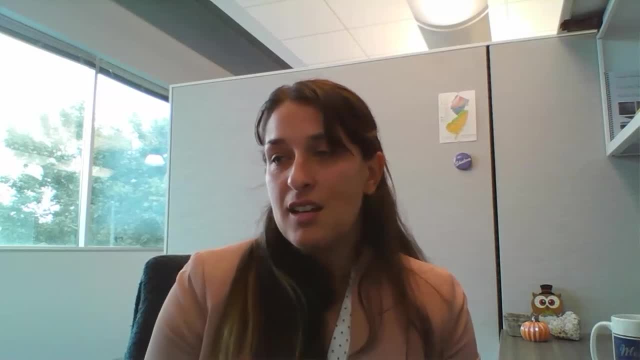 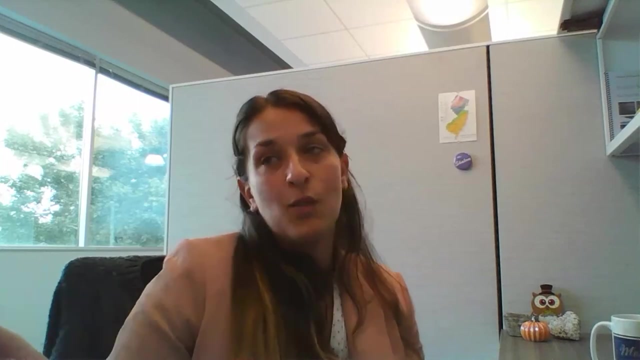 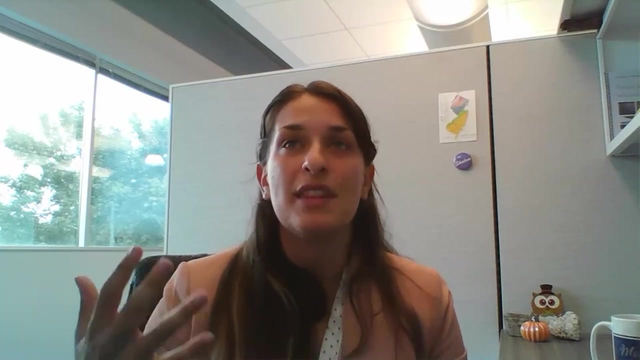 all right. so i think that, uh, some very difficult pollutants to undo are carbon dioxide, right? so when you emit it from burning fossil fuels, um well, actually even even other sort of emissions can just stay for a long time in the atmosphere, and so even if you've emitted it, 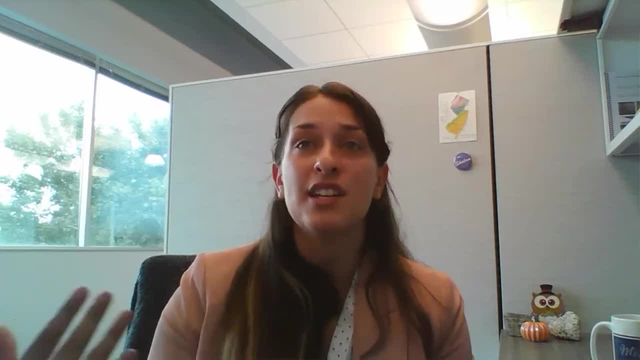 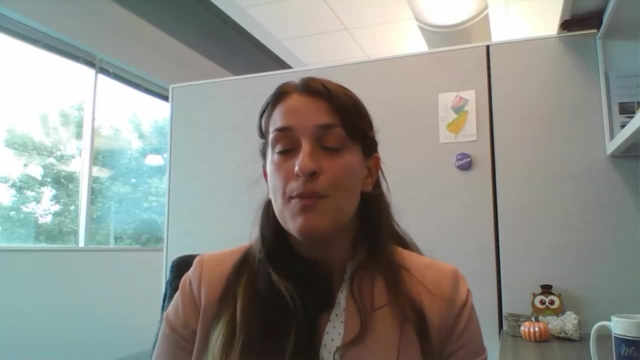 50 years ago. you're still dealing with the impacts years and years after that. um oh, and there's a very there's a new emerging contaminant that's come out that we've been finding everywhere and it's a very harmful effects and it's called pfas, which is 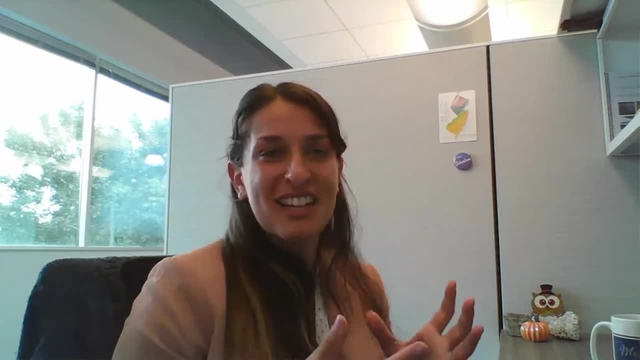 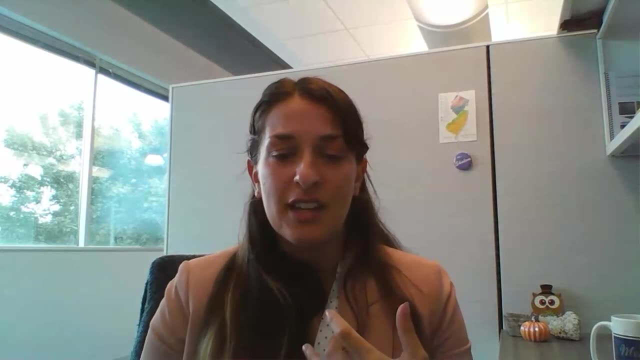 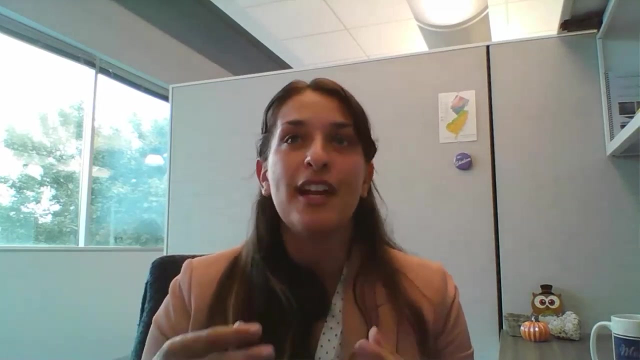 her fluoro. i am sorry you can't quote me on that, but there are all these different kind of per fluoro type of chemicals that are found often in teflon or sunscreen. they're found in all different sort of everyday products that we use and it's a new emerging contaminant where actually i'm going. 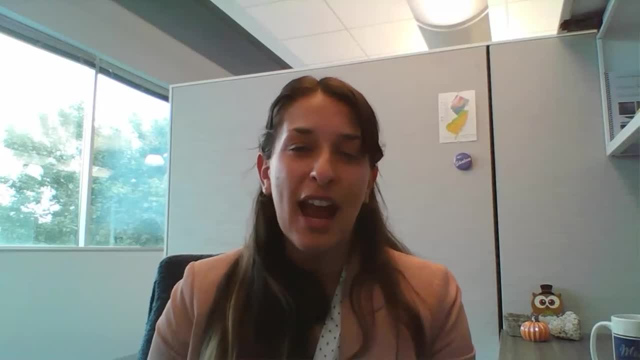 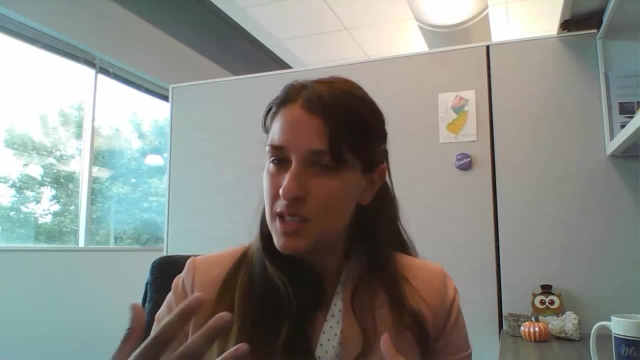 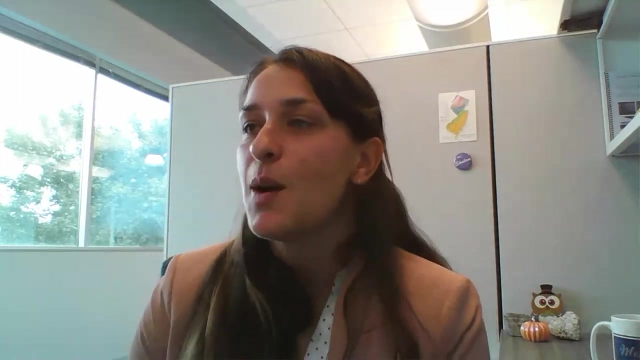 to a site on monday to sample for it, and we don't even have set rules and regulations yet, because it's such a new contaminant that we're still understanding and developing standards. for all right, let's see. all right, let's see what else there is. so how can groundwater contamination be cleaned up? 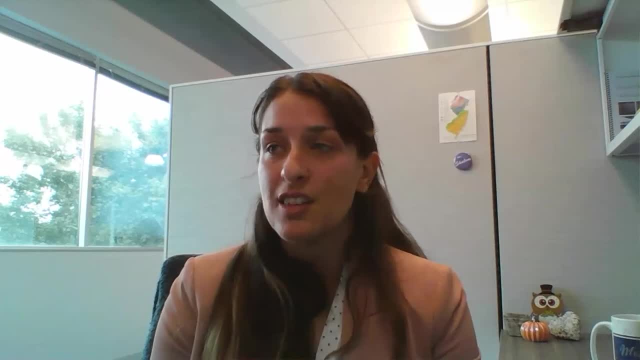 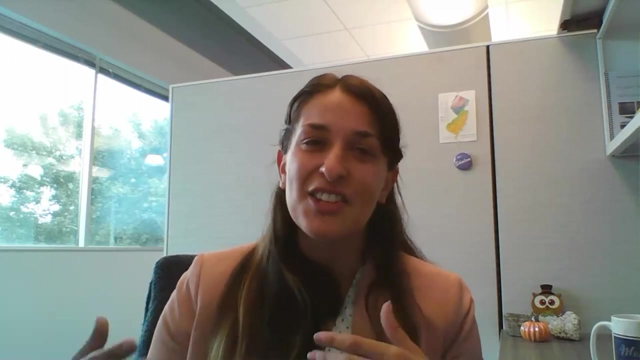 all right. well, there are a few ways- there are many ways actually- that groundwater contamination can be cleaned up and um, and one way that people do is called, like natural monitoring and, to summarize, it's kind of the solution to pollution is dilution and that over time, if you have some contamination in an 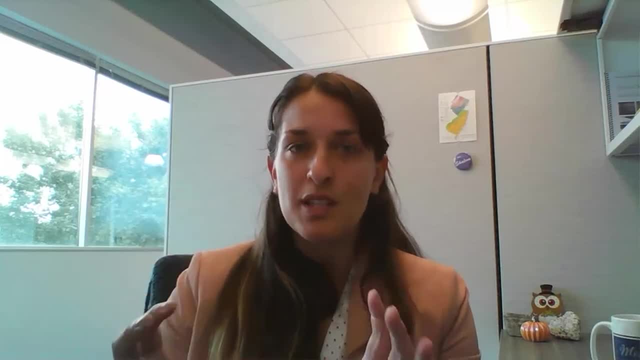 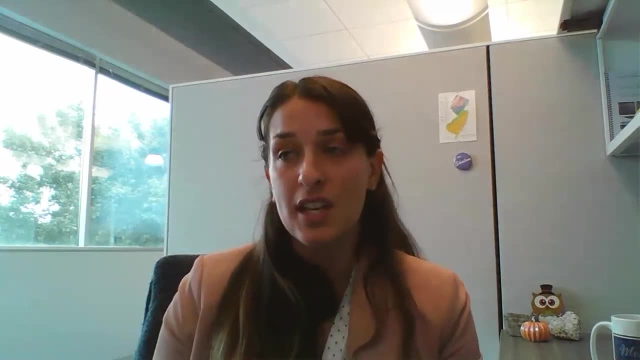 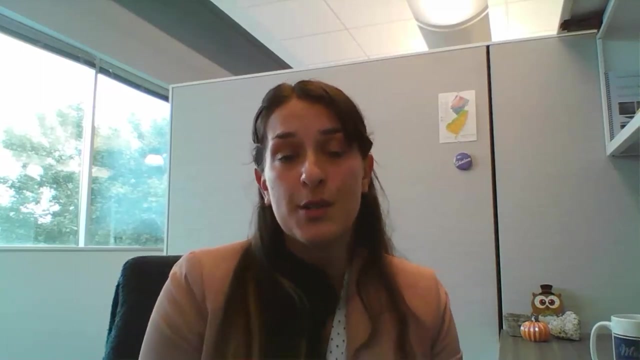 area and you block it out underground like that plume i was talking about, you sort of delineate the extent of it over time. when it gets diluted with more water, it can naturally mitigate itself, but there are technologies that can be used to clean up ground water. so, for example, there's a site in 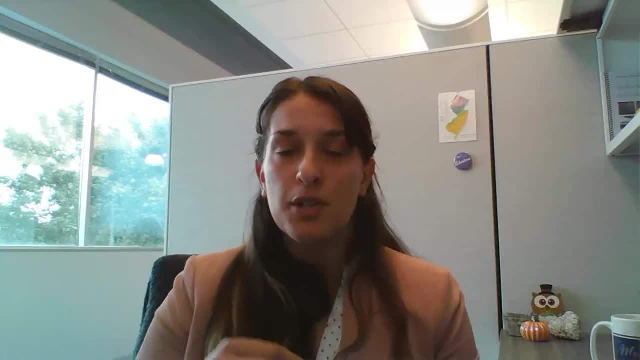 newark, new jersey, where there are a lot of petroleum related contaminants, and the way that we are cleaning them up is, rather than pumping that water out or just letting it dilute over time because the concentration is too high for that, What we do is we actually inject different nutrients, like bugs that will 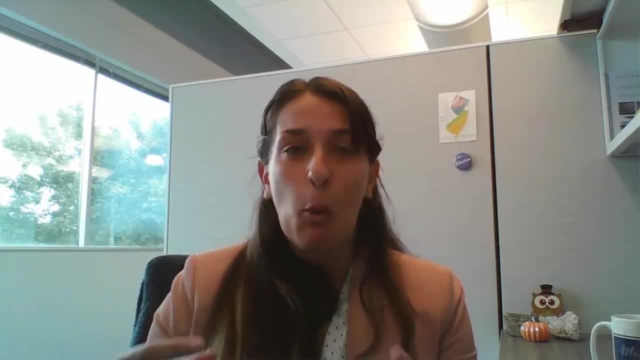 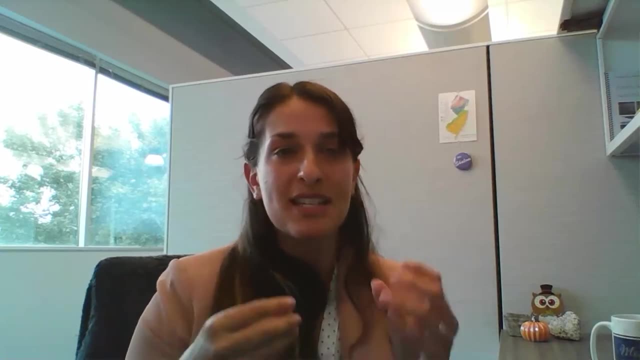 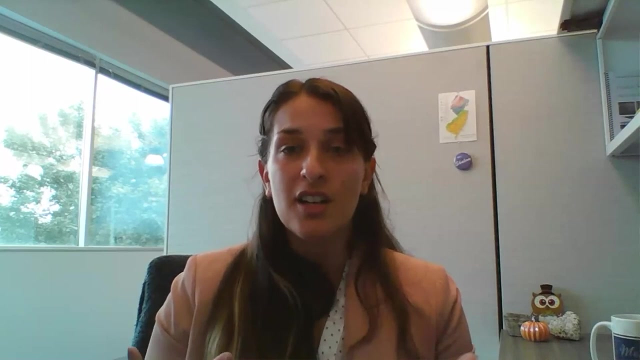 basically eat up that oil and stuff and naturally remove the contamination. So that's what we've been doing in injection: We mix different nutrients with water and we pump it into the ground and then we monitor it to make sure that the water is getting cleaner. All right, what else is there? Okay, 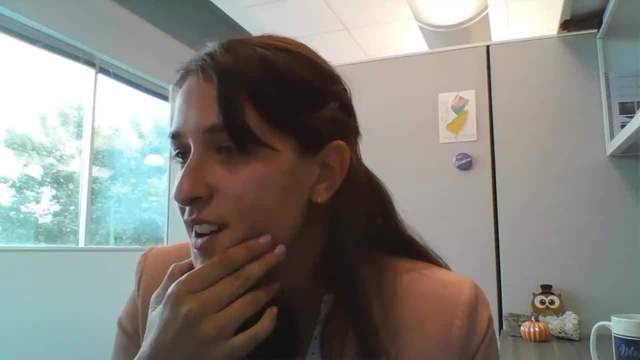 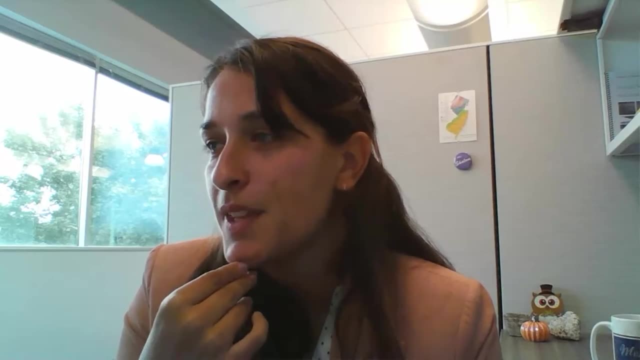 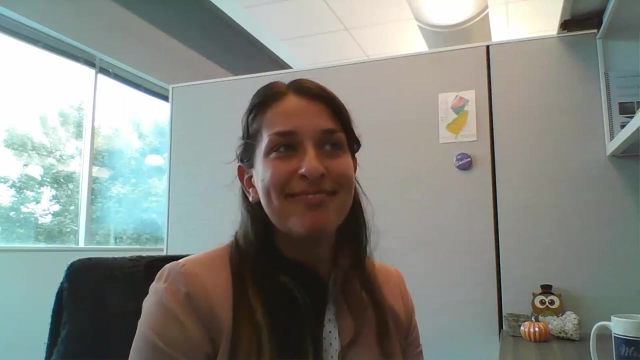 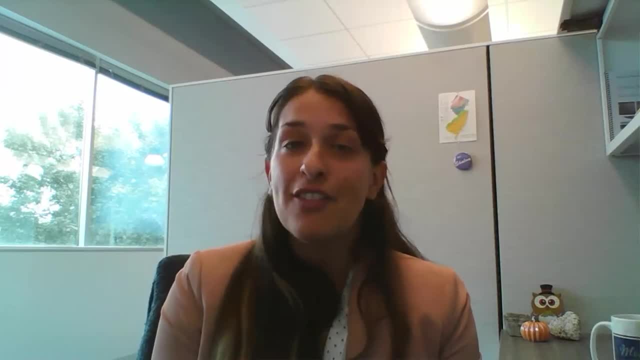 I don't have the most experience, but from my experience I definitely see a lot of those volatile organic compounds which are in cleaning solvents. They're in degreasing processes that a lot of industries use, and also a lot of, a lot of petroleum related contamination is what I see. 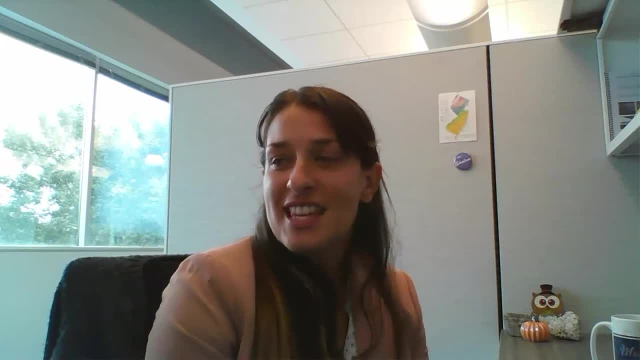 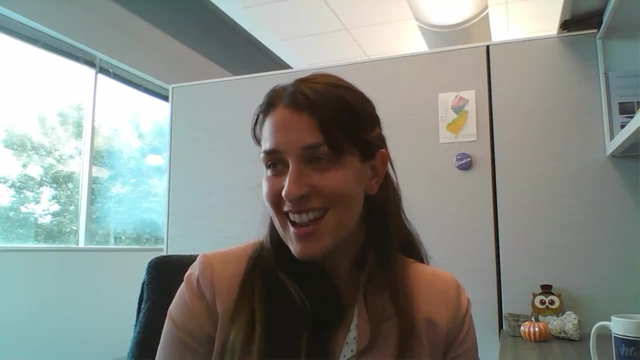 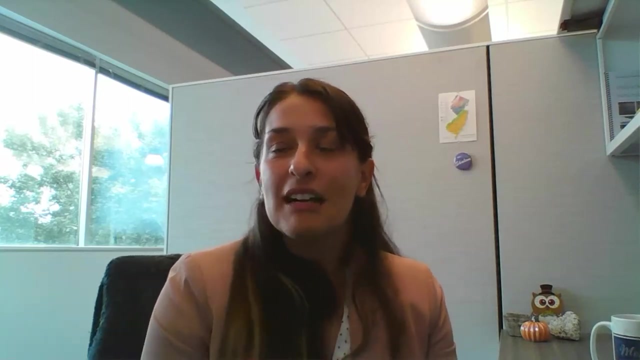 Okay. Michelle asks what is the tipping point and what technology is being developed to absorb carbon dioxide. Well, thank you, mom, for that question. So the tipping point- I don't know offhand what exactly it is- I assume you're asking for carbon dioxide. What's the amount of concentration that we can have in the air? 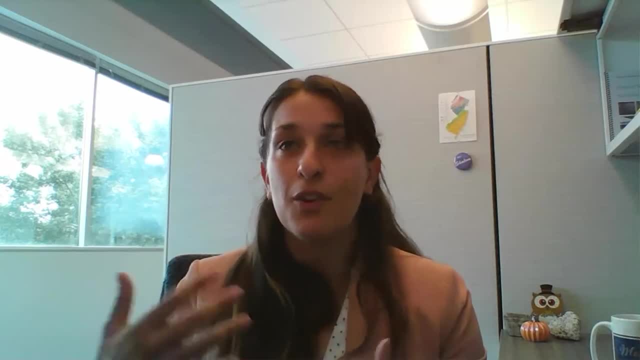 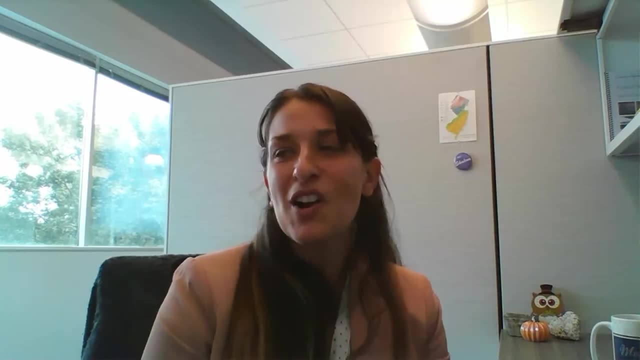 for reversing it to be impossible or for adapting to that to be impossible. I don't know exactly what the estimates are. I don't know exactly what the estimates are. I don't know exactly what the estimates are off the top of my head, but I think right now we're at like 400 parts per million. 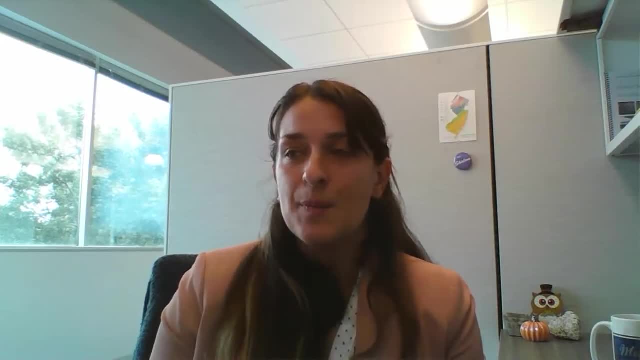 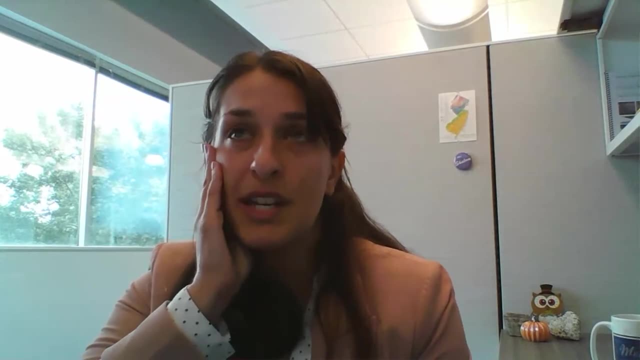 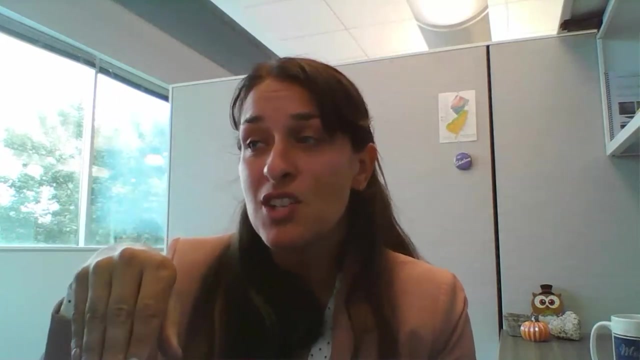 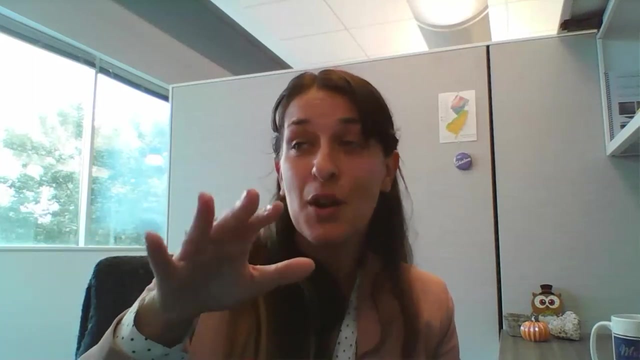 of CO2, and we're already estimated to probably go up at least a degree or so by mid-century, and I think, if we keep business as usual, it certainly will warm the earth at levels that we won't be prepared for. But the tipping point, that's a good question. I forget. I don't know exactly. 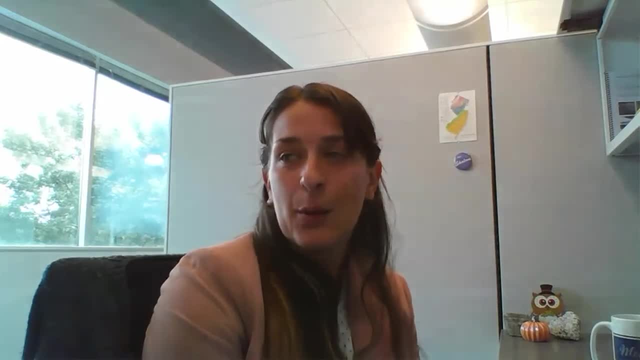 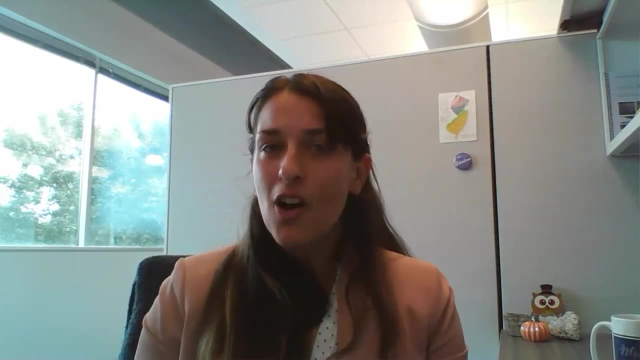 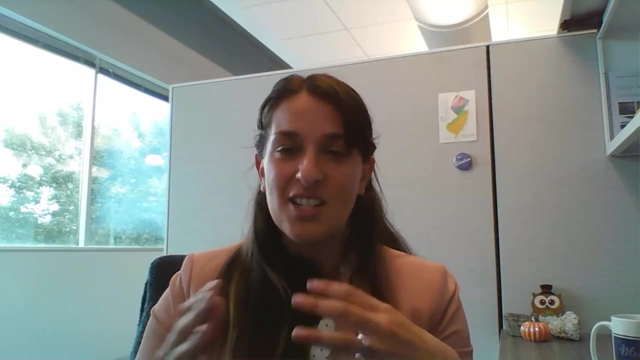 where it is- and I'm sure that it's also heavily debated- exactly where it is because it's not a clean-cut number. There are so many small processes that are involved and it's not just causation and fact. It's like a domino effect, where one thing will affect another thing and 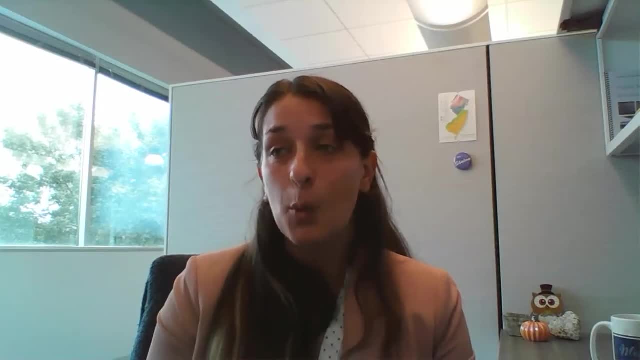 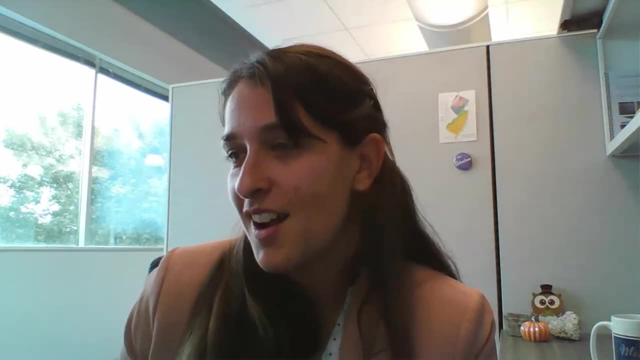 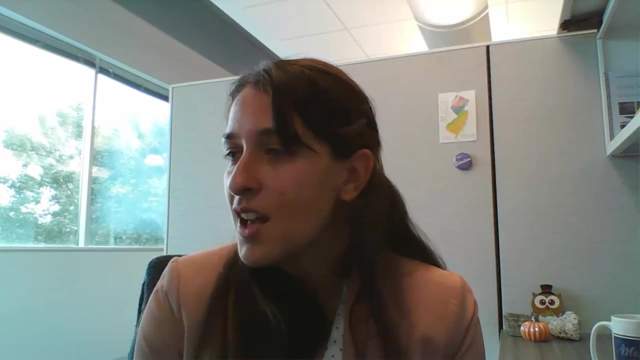 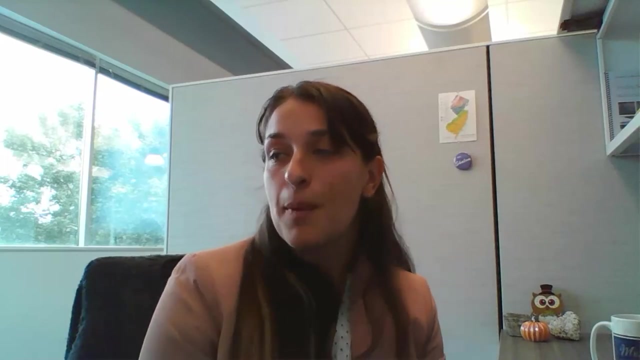 it's a very, very difficult subject to predict. All we know is it's definitely happening All right. Rhea's mom would like to know. I saw last. I saw last year or the year before in the summertime that there are a lot of dead fish watch washing up on the Jersey Shore. What caused all these fish to? 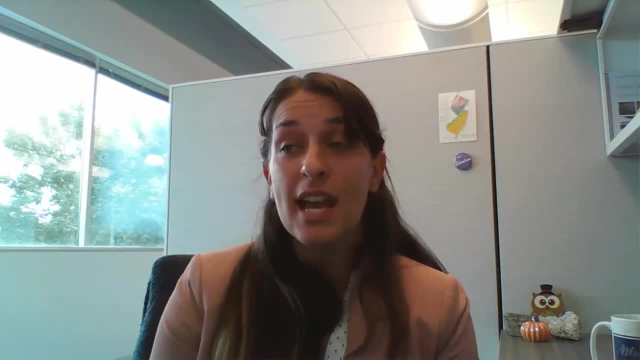 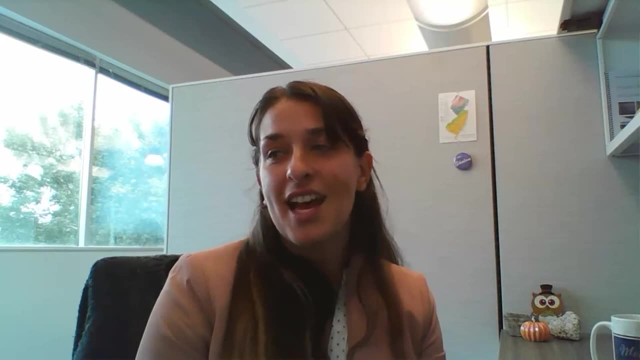 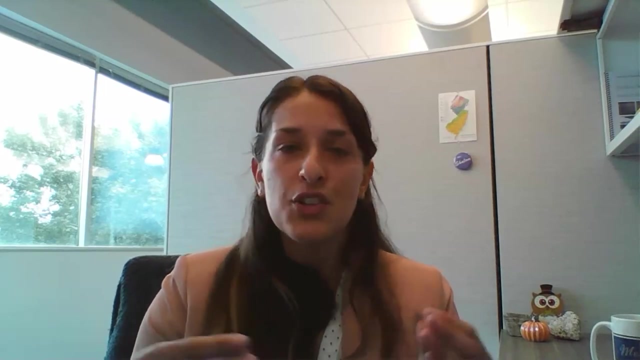 die. So, once again, this specific incident, I'm not sure, but if I were to predict, I would think that there was a lot of dead fish. There's a lot of dead fish that have died. You know, as I was describing with the last question that I think you asked, when you have all these nutrients that are. being added into the water. while nutrients seem like a good thing, right, because the algae in the water will want to eat it up, It actually grows everything off balance. So when you have one organism that can out compete, everything else and all these nutrients that are added by that runoff. 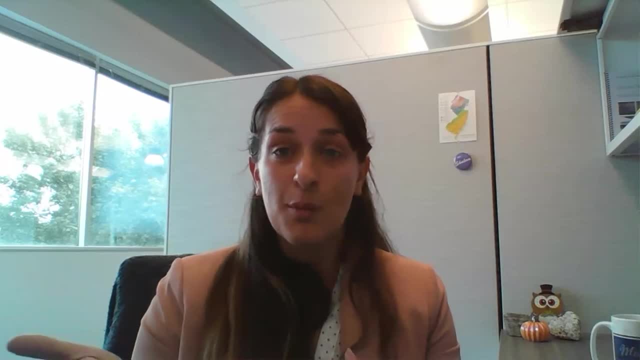 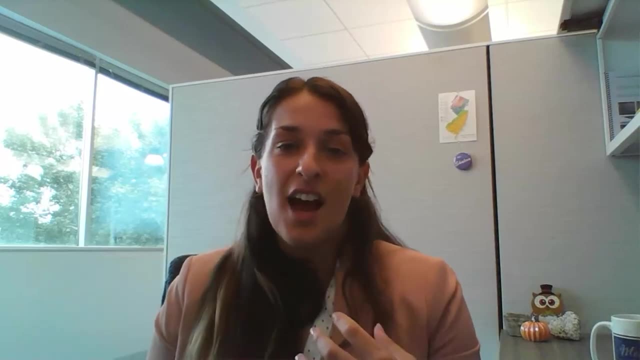 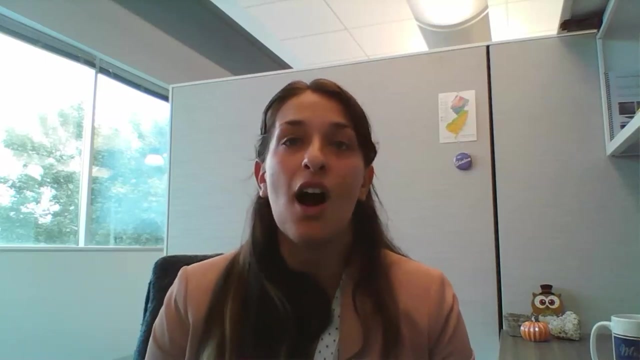 right going into the water, There's a population, maybe of algae, and then when there's too much algae and there'll be too much competition and then there could be a lot of death and and then you can get a lot of microorganisms eating up that algae and that can result in a change in the oxygen levels in the ocean's water and it can really mess up the equilibrium of the ocean's water and result in a lot of fish deaths. So I don't know if that answers the specific question. Pat Donahue says yes, there were very large oil spills in the Arthur kill many, many years ago. 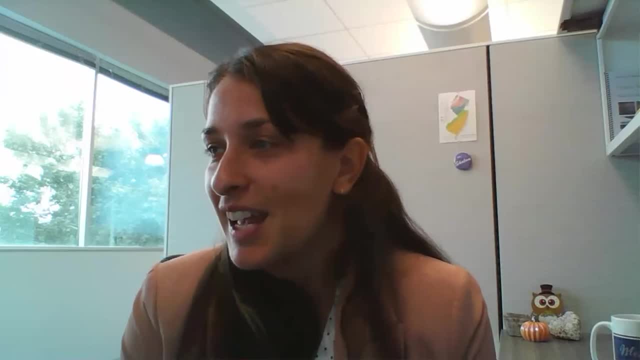 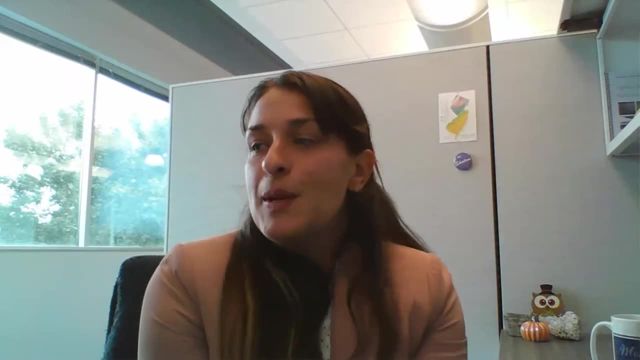 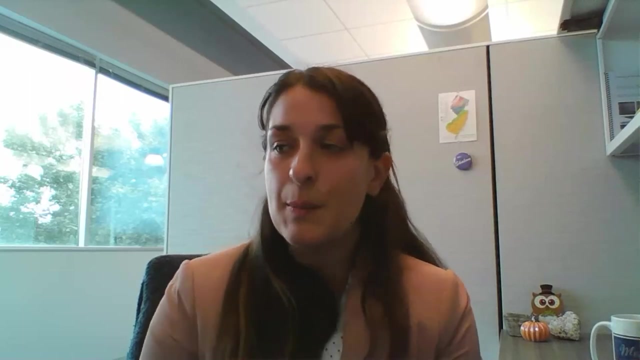 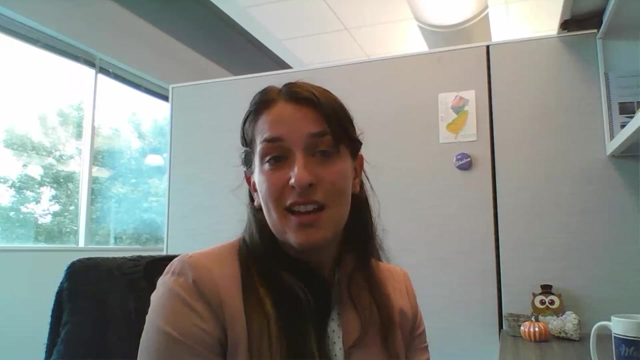 OK, Thank you, Pat, for letting me know What is the most exciting place that your research has taken you. I got to go through Rutgers with my professor, Gail Ashley. She's a geology professor, recently retired, actually at Rutgers, And I went with her to Tanzania. 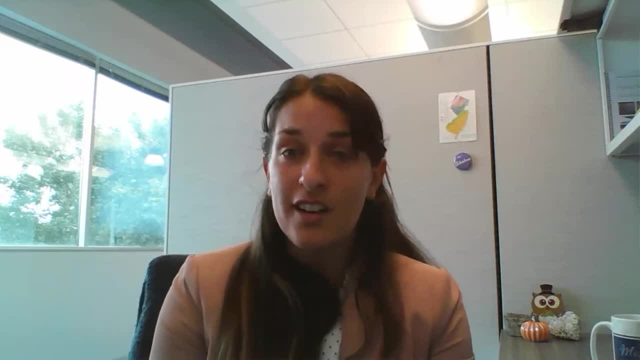 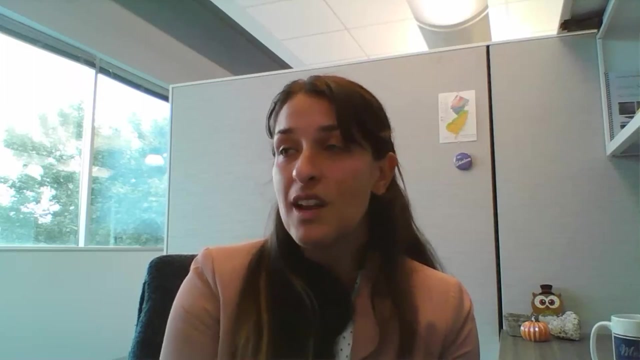 Africa to study groundwater there and we studied a lot of springs there and it's a very dry area but they have these beautiful springs that provide water year round and they really hadn't been studied. So we went there to study that and it was really amazing experience. 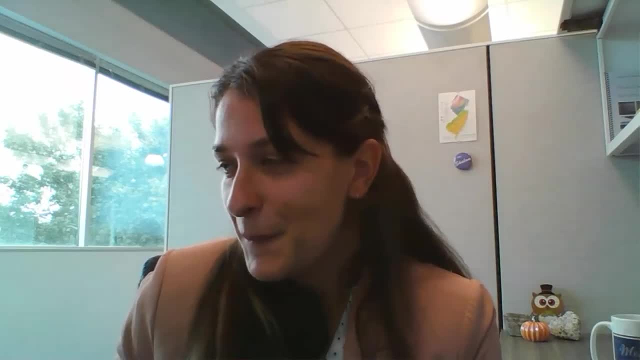 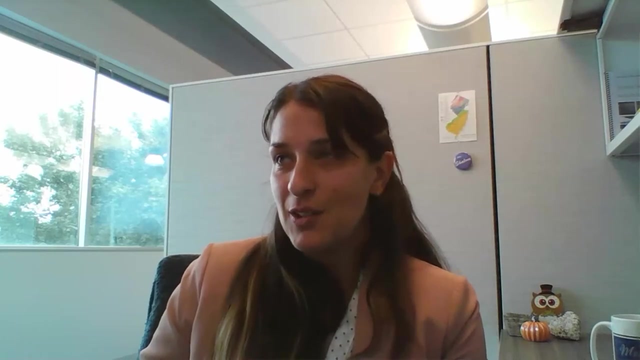 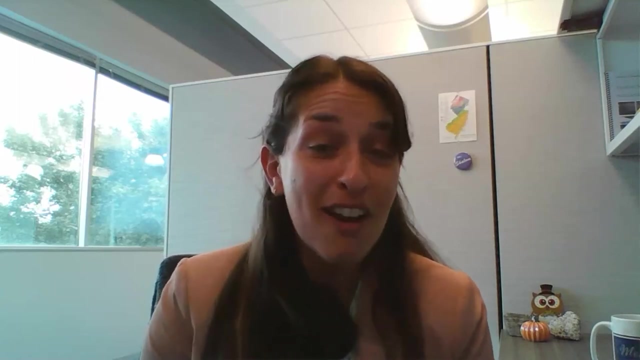 All right, Let's see. what else am I missing? Rhea's mom would also like to know: when you go out to do your field work, what types of wildlife do you encounter? OK, So that's a good question. She asked specifically: do you ever see snakes in New Jersey? 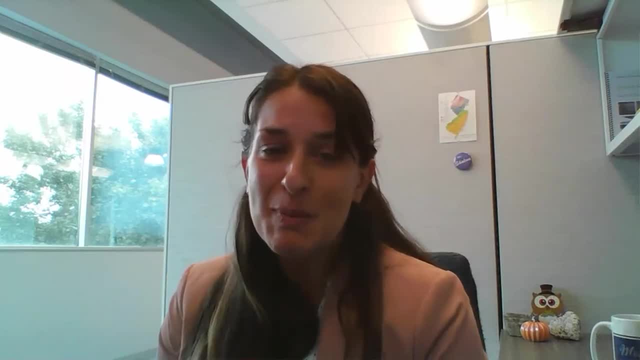 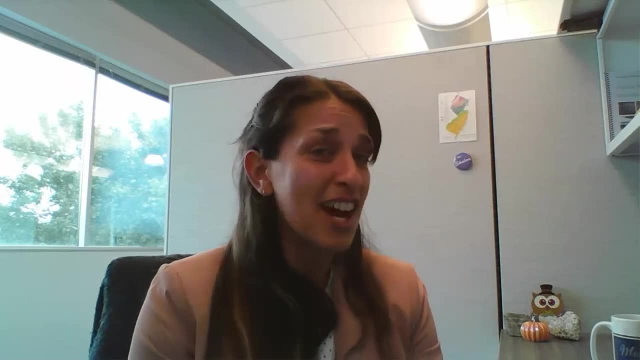 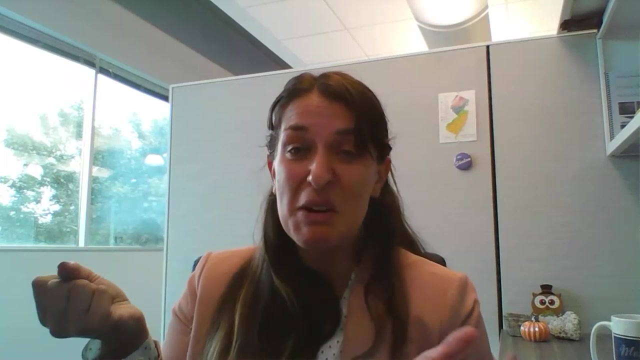 And I think I've seen like a garden snake maybe once, But I see surprisingly a lot of street cats in the areas that I'm working and they're really tough looking street cats, But Unfortunately, I see a lot of bees. sometimes when you open up a well, there are bees inside and really nothing amazing in terms of wildlife that I get to see. 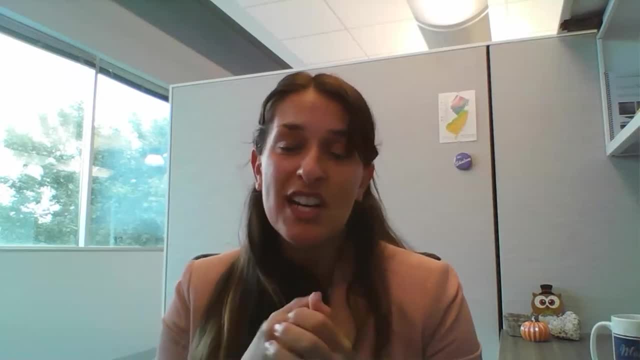 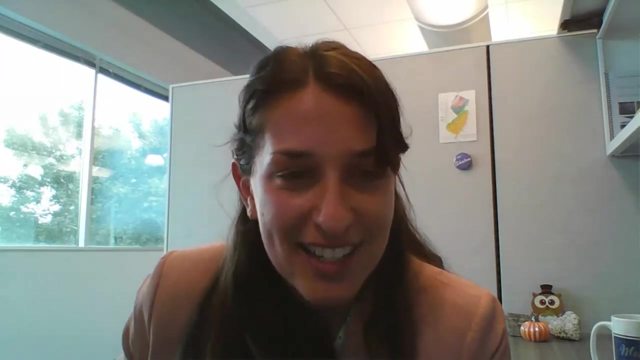 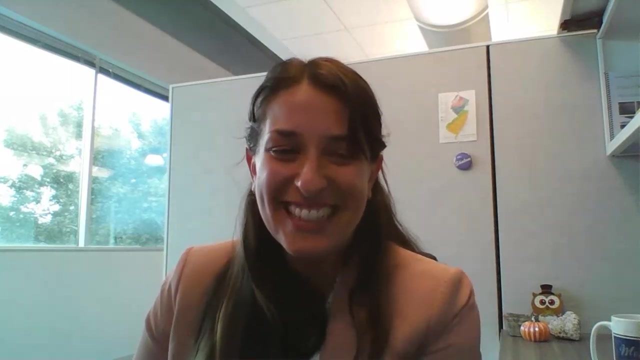 Because a lot of times I'm working in cities. sometimes I'll go out into a more, less populated area, but a lot of times I'm working in cities so I don't get to see the best stuff. All right, Let's see A lot of questions. 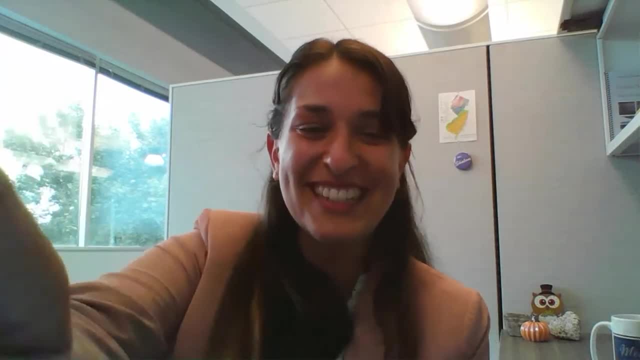 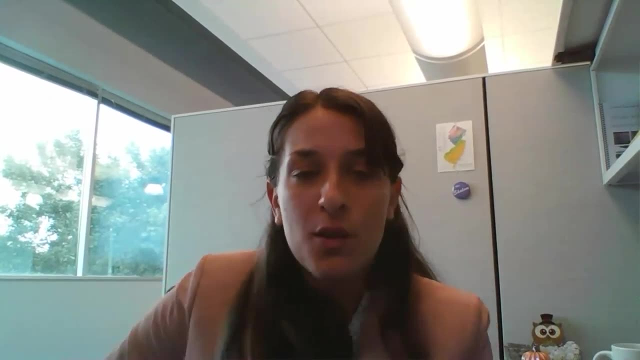 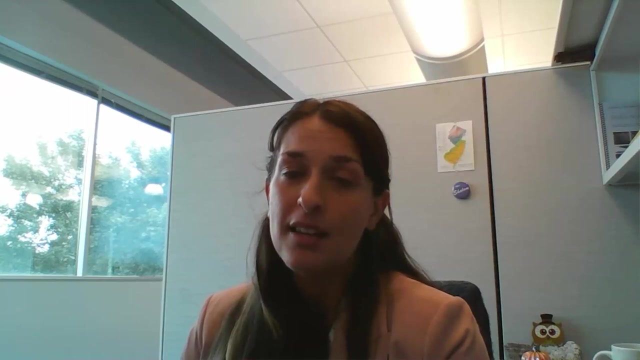 Really good questions, Some of them I can't really answer. OK, Ariel would like to know: do scientists agree on climate change? Do any say it's not real? So I think most scientists are in consensus that climate change is a real thing and it's happening. 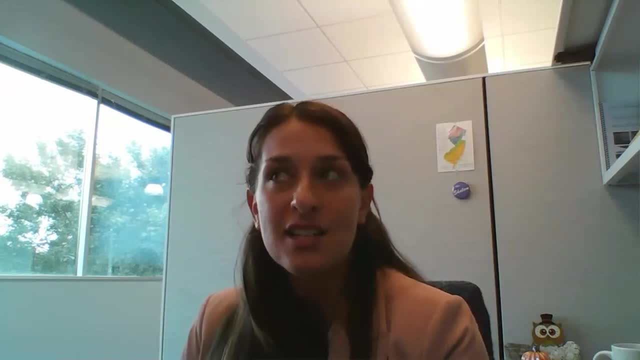 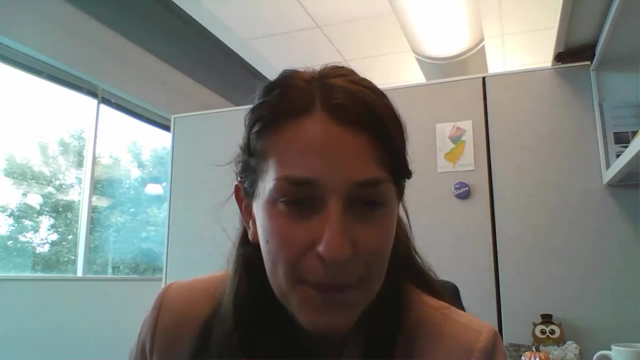 But there are definitely people and scientists who provide information to show the opposite. But there is most consensus- I think there is mostly a consensus- that it's happening. OK, Ariel also wants to know what's your favorite thing about being a geologist. 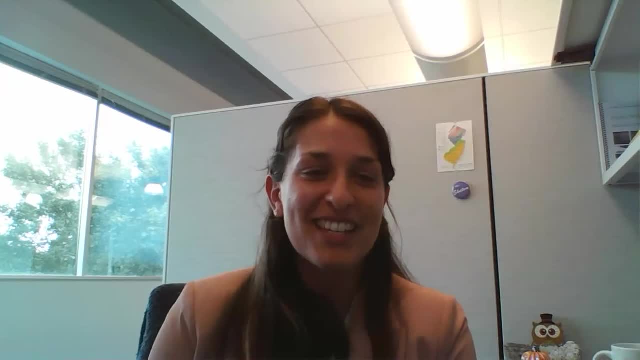 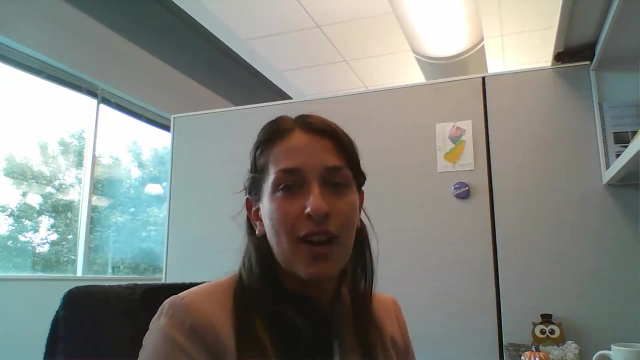 That's a good question, Ariel. So my favorite thing about being a geologist Is a. it takes me to really awesome places and in the field where you get to see, you get to travel and you get to see new and different kinds of environments. 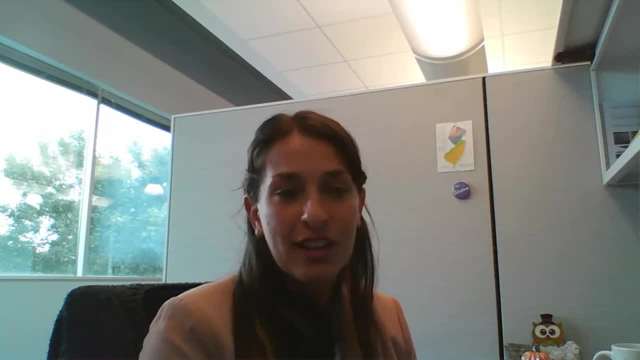 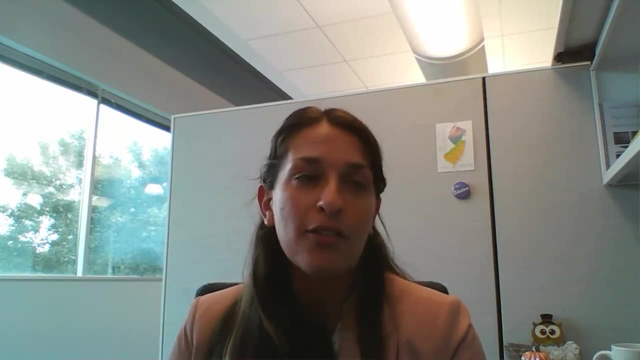 And also, what I really like is that you can be very curious And if you have a question, geology is all about finding the answer. So you can continue to be geologists and say, well, well, why is that there and why is this happening that way? 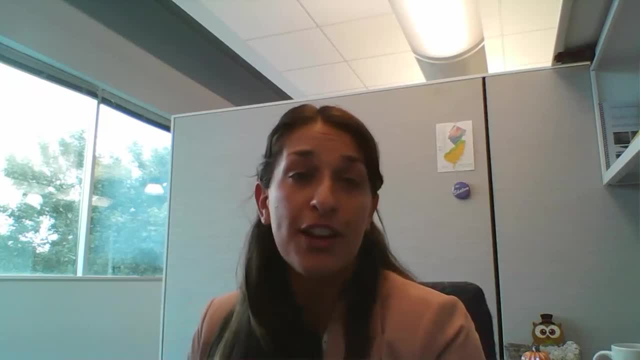 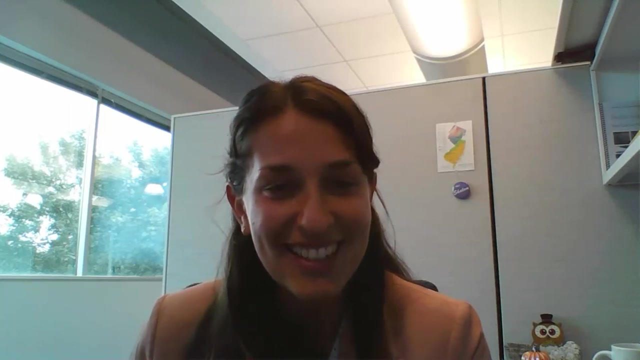 And then you get to come up with a solution to figure out the answer, And it's very hands on like that, And I think that's what I like most about geology is. it satisfies my curiosity. All right, What test or instrument would you like to invent for your work? 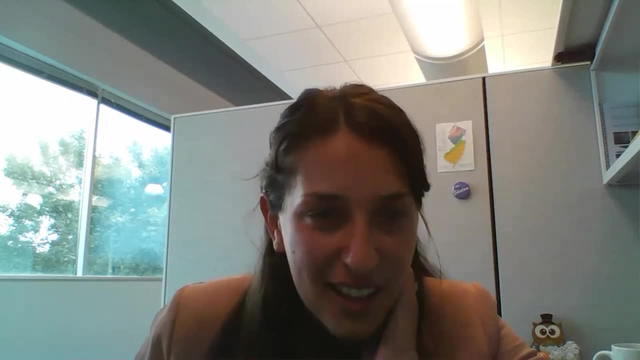 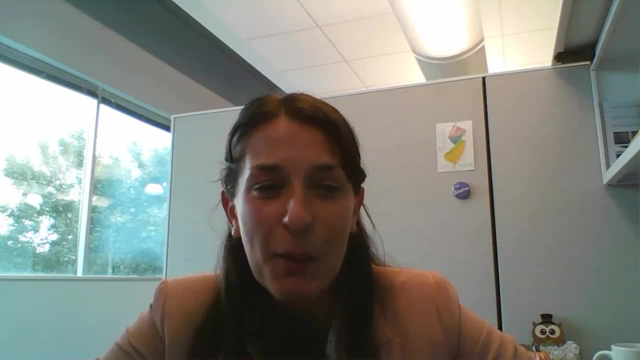 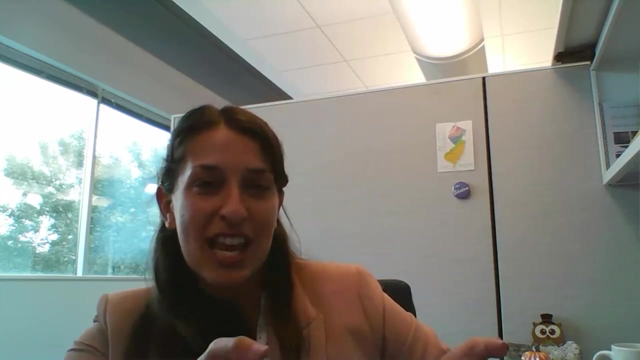 That's a fun question, I think. Who asked that? Mary, again from Scotch Plains. So I think if I could come up with an instrument- I have no idea how this would happen, but I don't know if you all are aware- with Shazam, which is like something you can, an app that you can use to identify a song if you don't know the song. 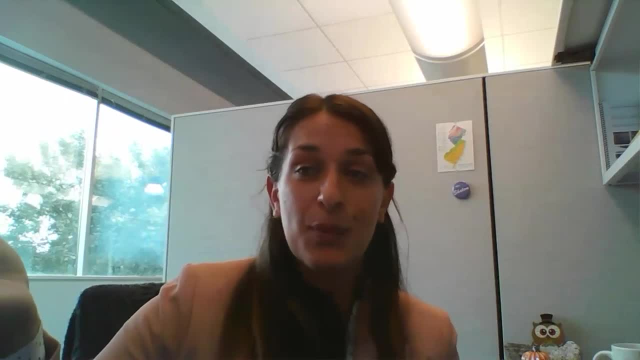 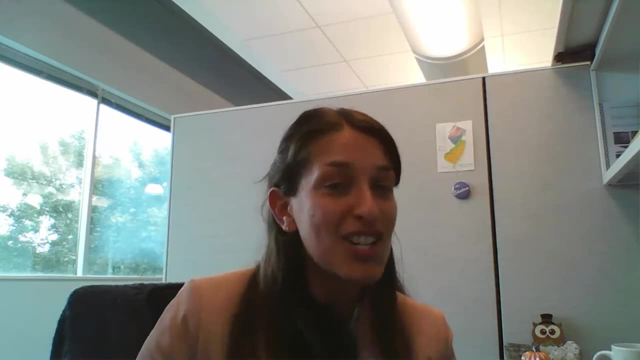 And I know they have made like the same thing for plants, where you can take a picture of a plant and it'll identify what planet is for you. But it would be great If they had Shazam for contamination, Which is like expediting the whole lab process. 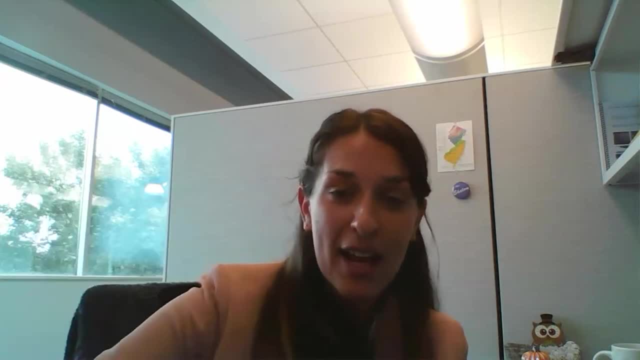 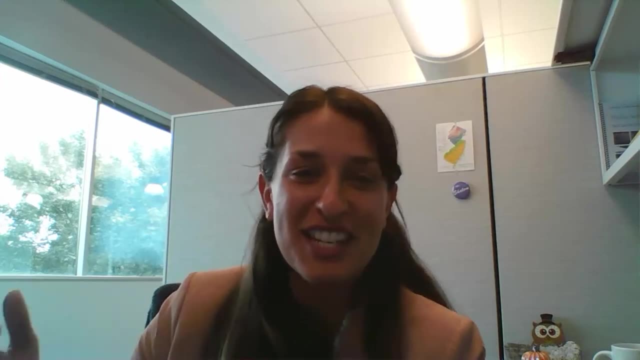 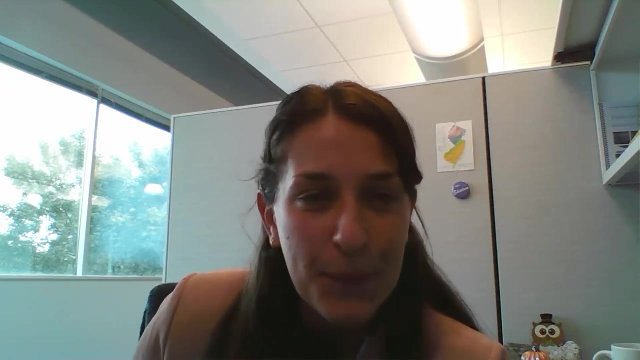 It would be great if you could just take a picture and maybe could identify exactly what soil you're looking at. That would be kind of cool and tell you if it's contaminated, what kind of contamination. but that's kind of fantasy. All right, Can I test for air and water pollution at home? 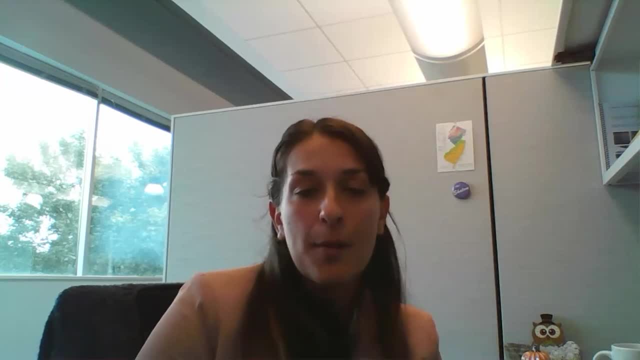 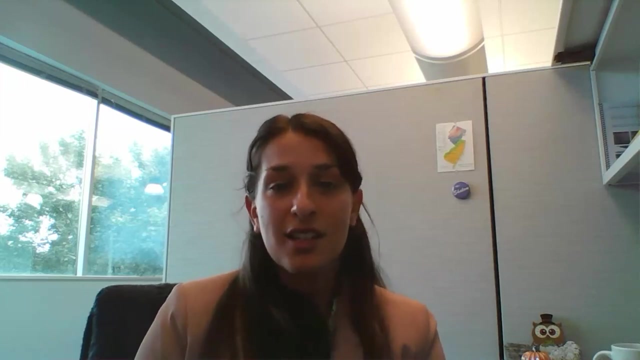 And how. I know that if you, if you have your own well, you your own well water and if you're not, don't have public well water or you can probably just grab a sample, You can buy a kit to collect a sample. I know that sometimes the town will send water reports. 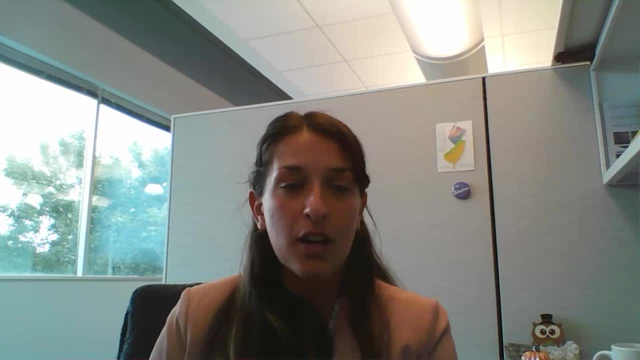 But I'm pretty sure that there are companies that you can hire to test the water in the air for you And, while the firm that I work for is usually for corporations and at a larger scale, we definitely do it And but there are definitely ways that there are kits probably you could buy for testing your own water, for example. 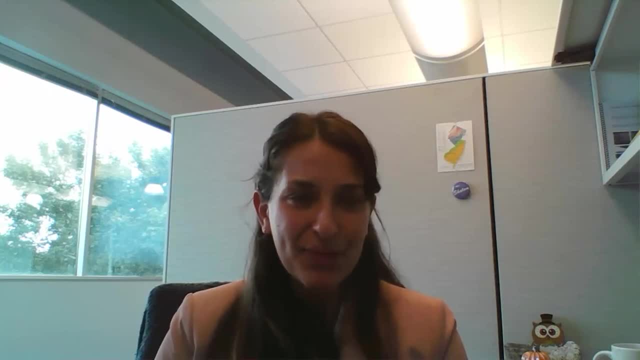 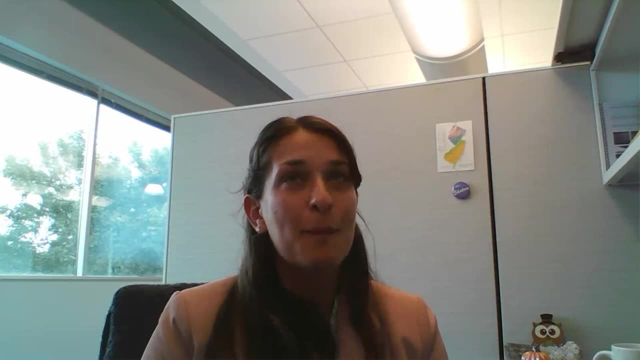 I'm not at familiar with what it is. Can I remove microplastics from my water? That's a really good question, And I don't know, Because they're supposed to be so small. you can't see them, from my understanding, So I don't know how you would filter that. 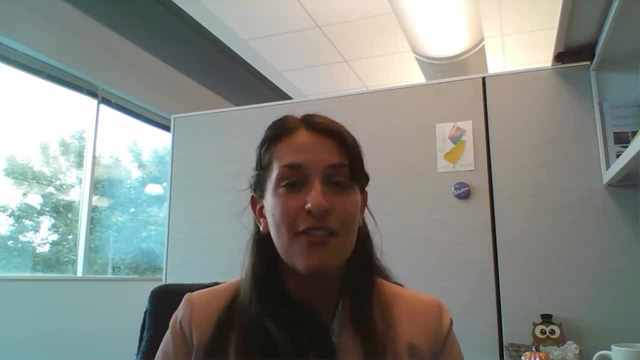 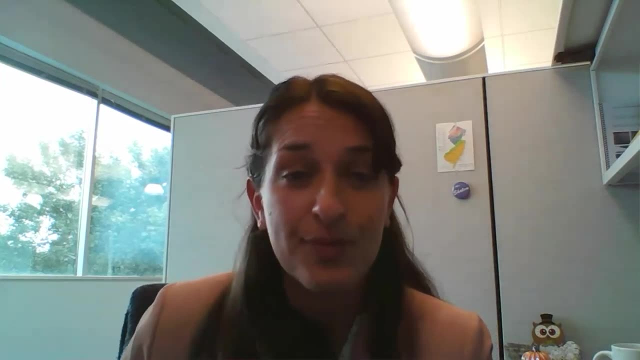 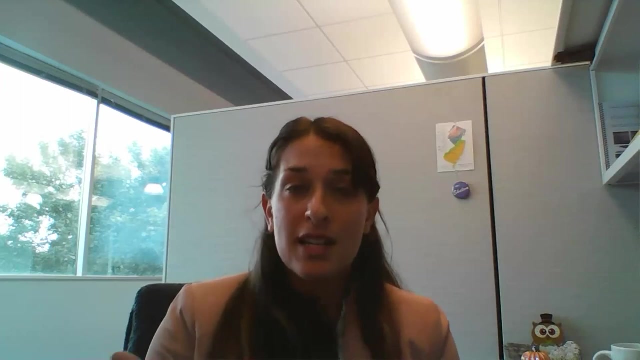 So that's a really good question and something that is definitely a concern. So next question, Mary. So what should I ask my town or government to prevent or clean up pollution? So, as I spoke about earlier in the presentation, That there's this new initiative in New Jersey and a new policy to move away from using plastics. 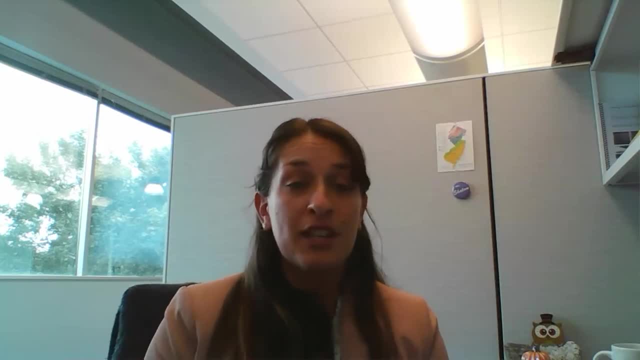 That's definitely an example of something that you can ask your town or government to do, Which is, you know, if you live in a school, maybe you can figure out how much those water fountains are, that you don't have to press the button, It'll just refill your water bottle for you. 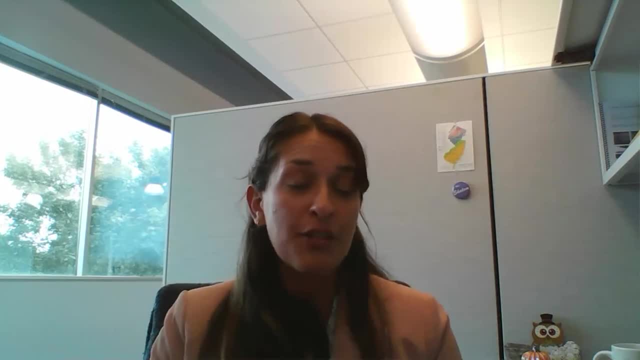 Because those save water as well, And if you can advocate for installing those in your school, that would be a cool idea. What else Do you work? in- urban areas or more undeveloped places? I work in a mixture of both. Sometimes we'll work in an area that hasn't been developed, but they want to develop it. 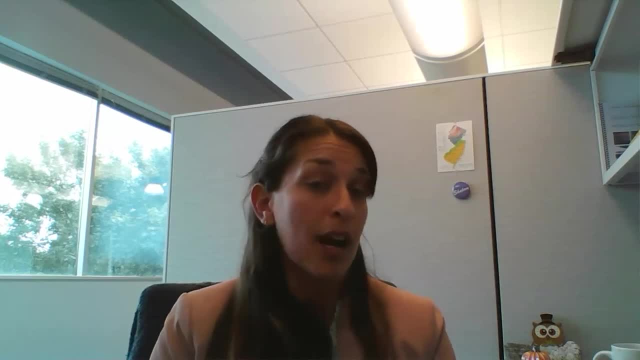 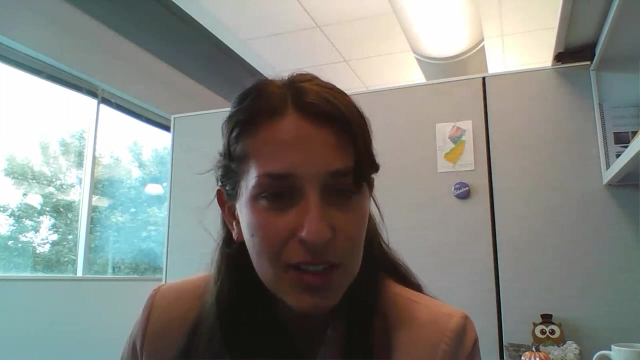 But first they want to check if there's any sort of an environmental concern. But mostly my experience is in more urban areas Because, as you saw from that geo web slide, There's just a lot of contamination there. Alright, What else? What is the oh wait? 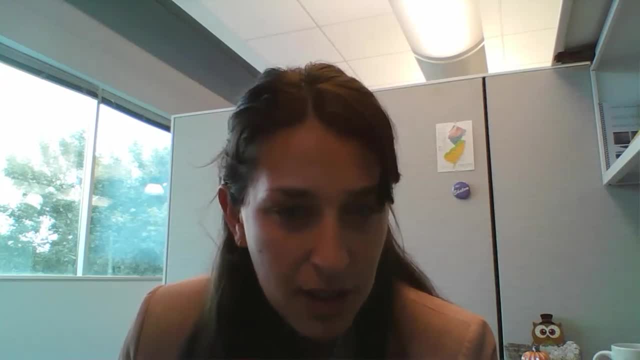 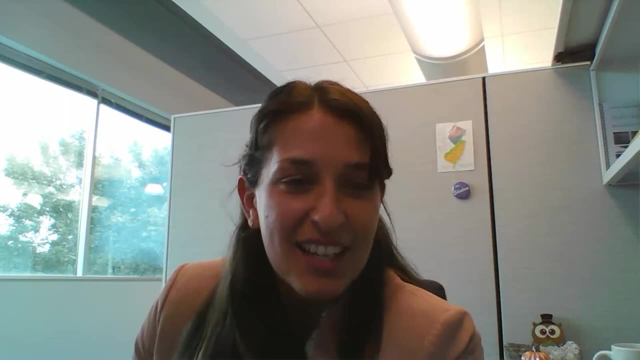 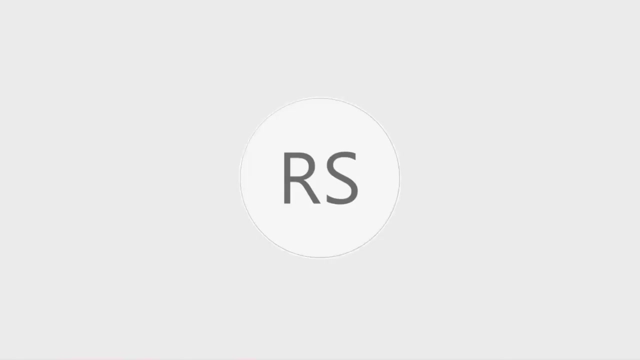 Alright, just looking through the questions, The ones that I've answered. Ahem, Sorry, Monica. No, it's okay. There's one more question for you. Do any other fields help you in your work at Roo? Any other fields help me in my work at Roo? 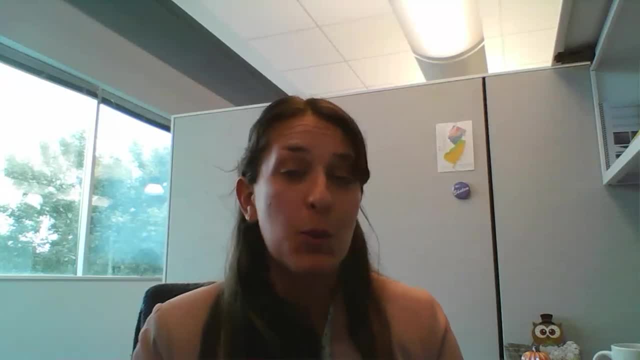 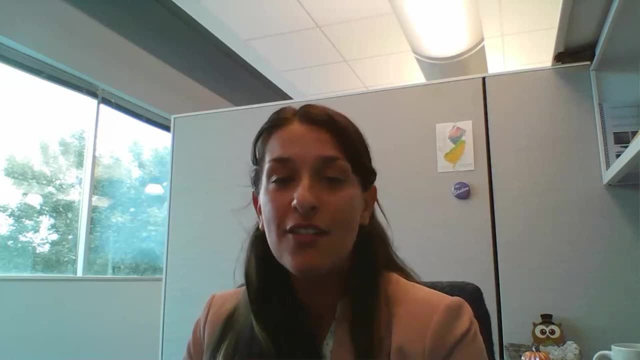 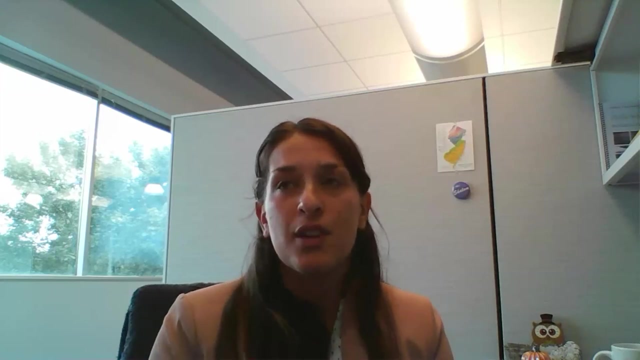 Like if you mean different sort of subjects of study that might help me in my work. So geology definitely helped a lot. Ahem, So other sort of- let me think, other sort of fields that are helpful were, if you did any sort of engineering. 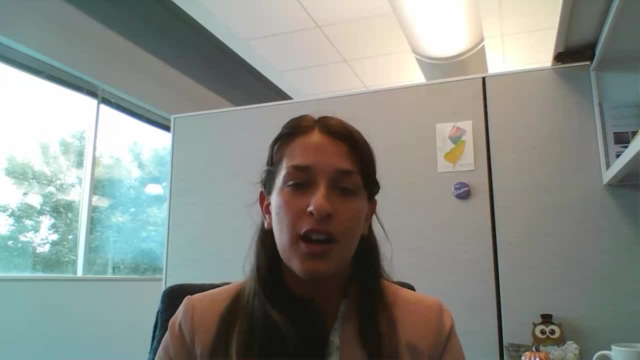 Because a lot of the systems that are created are engineered systems to remediate, to clean up contamination. Let's see what else. So if you took chemistry, that actually is really helpful, Because there are so many chemicals that we have to learn about. 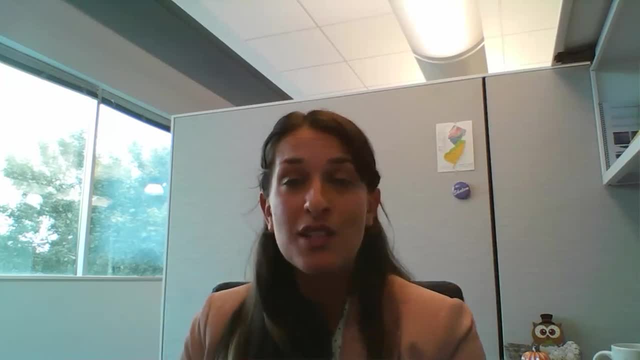 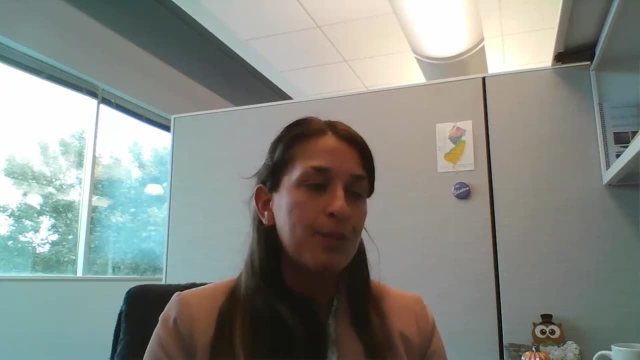 And they're a mouthful to pronounce, So it's helpful to understand. you know, even though we aren't a laboratory and we're not conducting the analyses, We get all the results back and we have to interpret them correctly, And so chemistry is definitely something that can help your understanding at Roo. 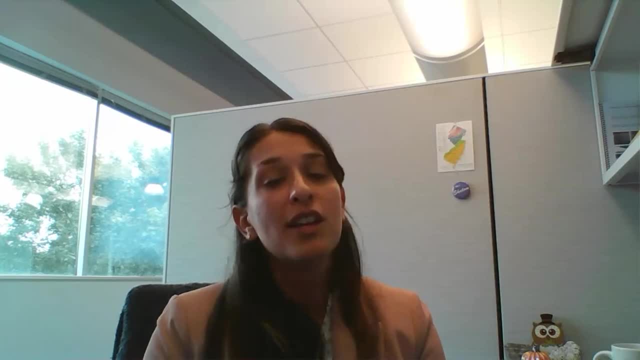 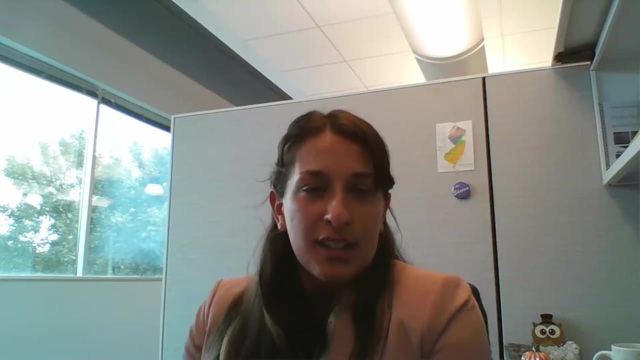 What else? Really a lot of what you learn, what I've learned at Roo. I learned at Roo, But having that geology background definitely really helped me understand things a lot better and ask the right questions. Okay, thank you so much, Monica.